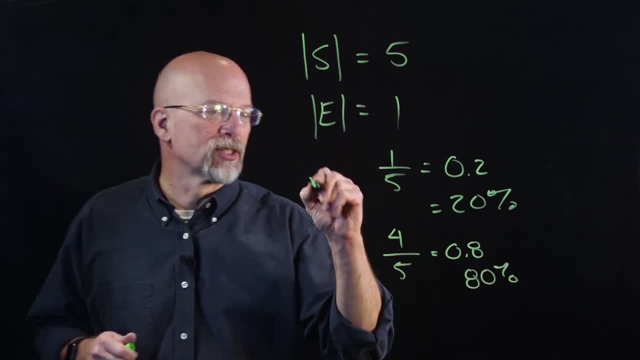 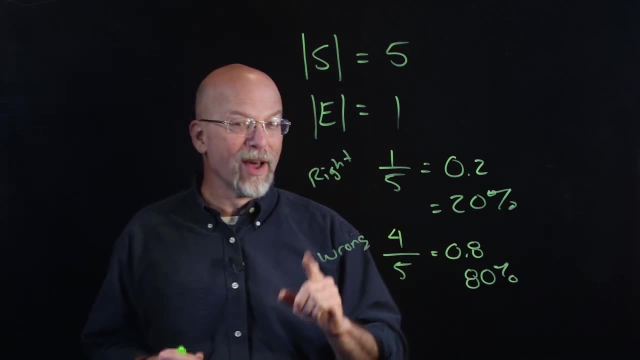 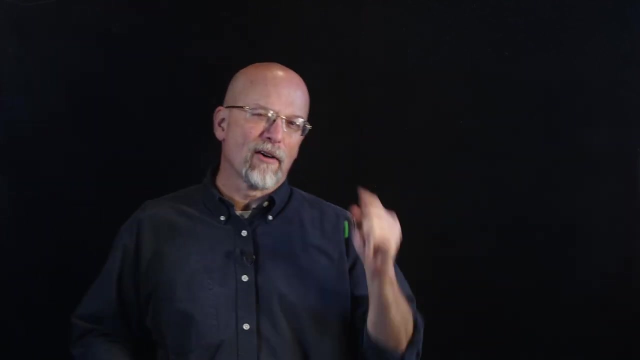 point eight or 80%. So this is right and this is wrong. But let's assume we have more questions than just one that we're going to have to guess. Numbers change a little bit. in that case, Let's work this out for two questions, starting with the first question. So probability of 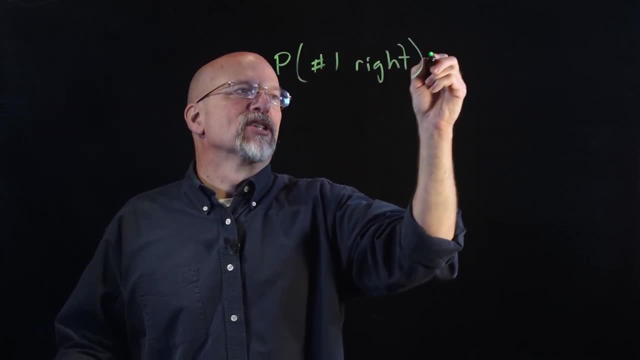 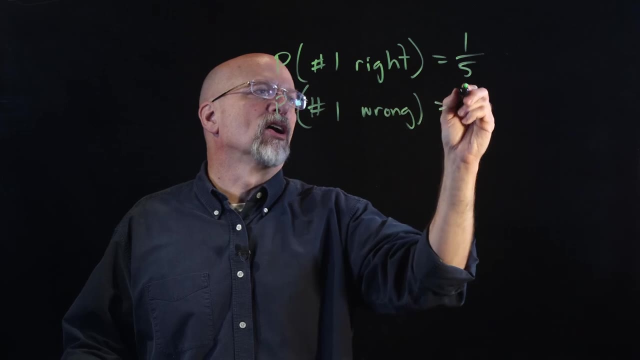 question number one is right, So that's just equal to one-fifth, right? The probability that question number one is wrong, that you guessed wrong, is four-fifths. Remember, there are five options for each one of the questions: A, B, C, D, E, F, G, H, I, J, L, M, N, O, P, R, S, H, I. 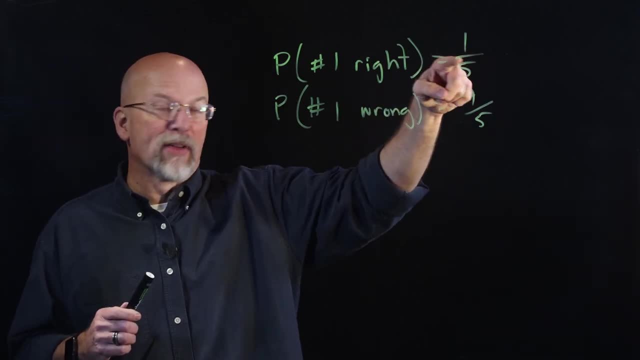 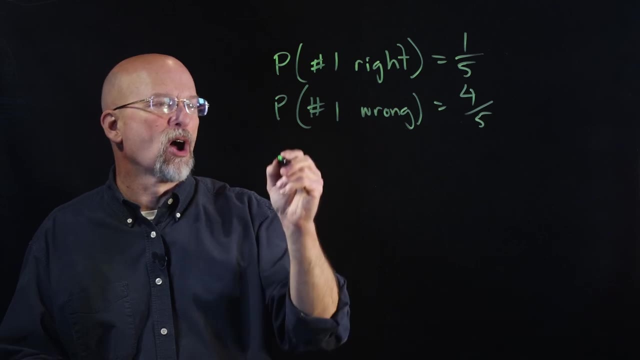 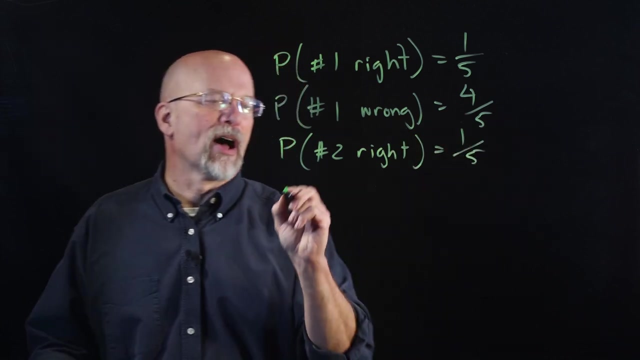 D E all right, And one of them is right. So you have a one in five chance of getting the right one, the one right for problem number one and a four in five chance of getting it wrong. Now we have a second question, problem number two. What are its chances? Well, one in five for being. 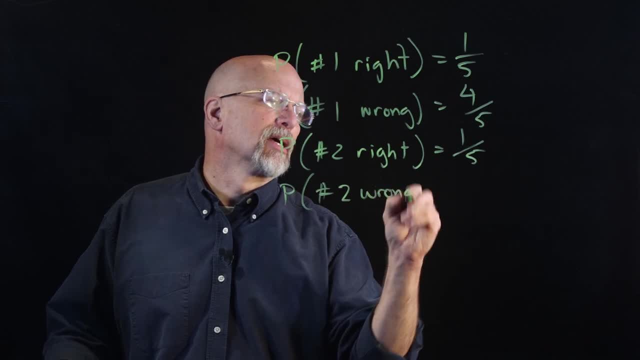 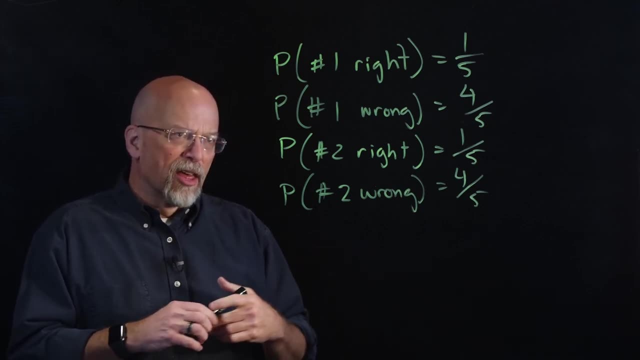 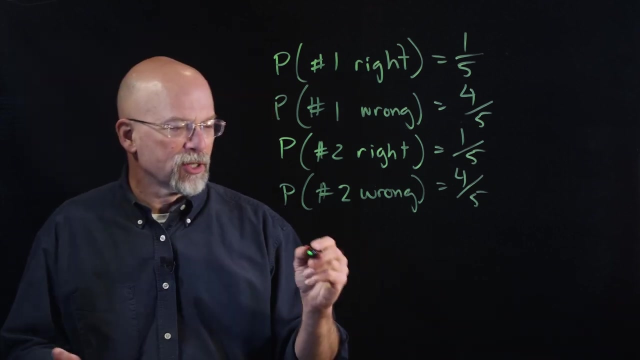 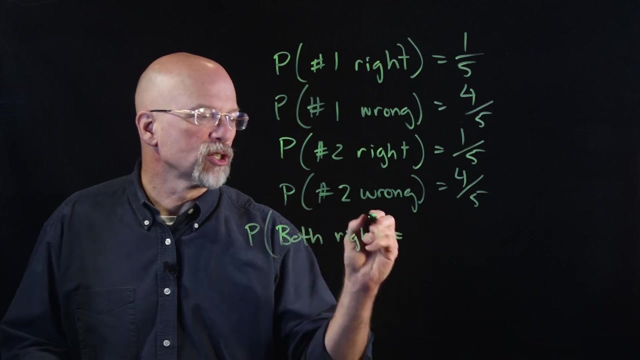 right and four out of five for being wrong. So what are the chances that you'll get the right one, that you'll get two right, or one right and one wrong, or both wrong. Let's take a look First of all. if you get both right, what are the chances? once again, we are just guessing. these are just 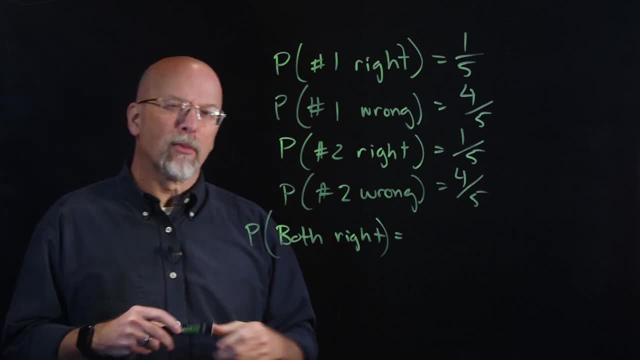 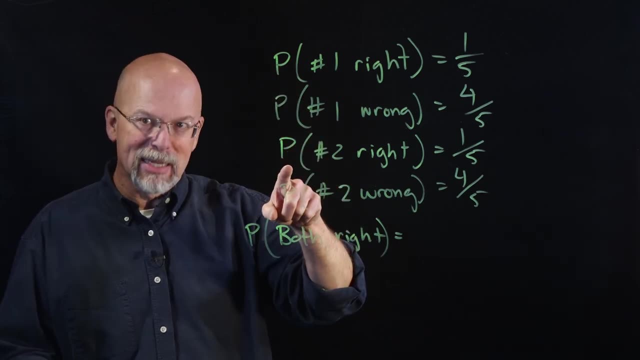 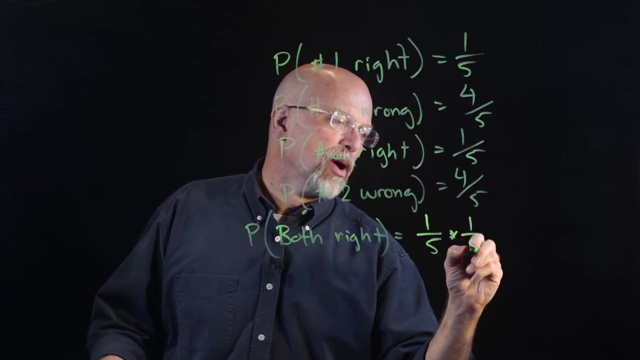 random guesses and to get both right. and, if you remember, we had this multiplicative rule for probability. so, that said, if you want to get number one right and number two right, you multiply those probabilities together so it becomes 1, 5th times 1: 5th, which is equal to 1: 25th, so you have a 1 in. 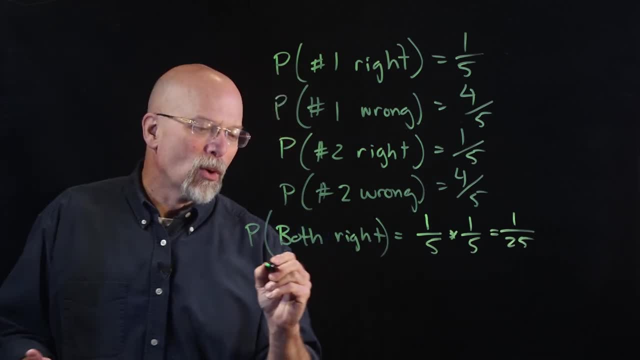 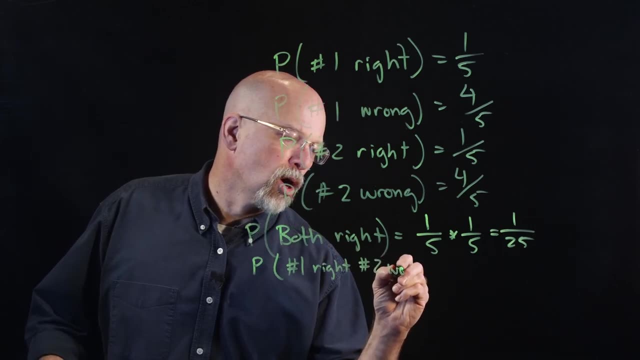 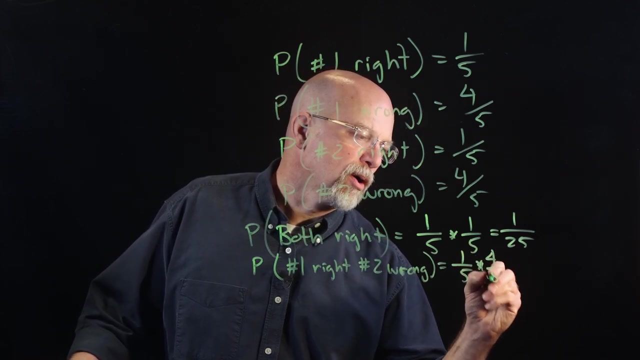 25 chance of getting both right. But what about the probability of number one right and number two wrong? Well, in that case, what you have is 1 in 5 times 4 5ths, which gives us 4 25ths. and that's 4 times 2, right? so that's 4 times 2, right? So that's 4 couches. Now let's take a look. 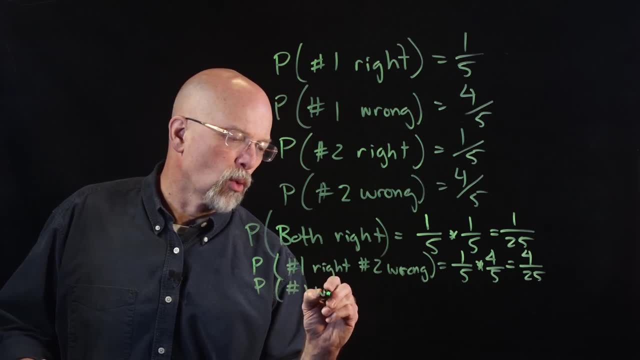 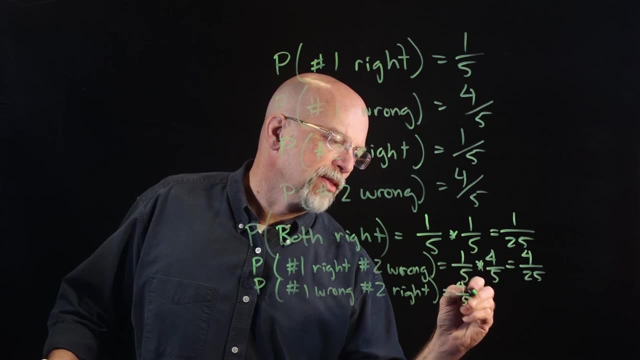 and we'll get four together, which gives us 4- 25ths. and then let's take a look at these probabilities And, similarly, if I'm looking for number one wrong and number two right, well, in that case we've got four-fifths times one-fifth, which also is equal to four-twenty-fifths. 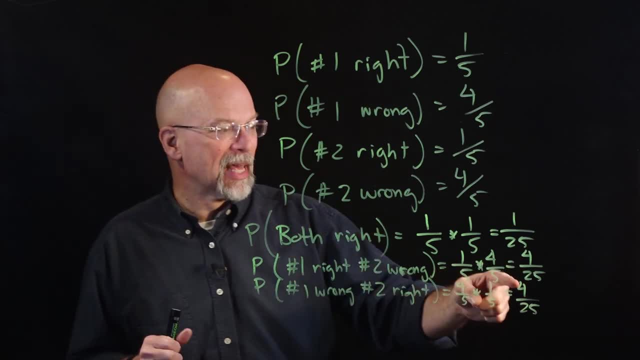 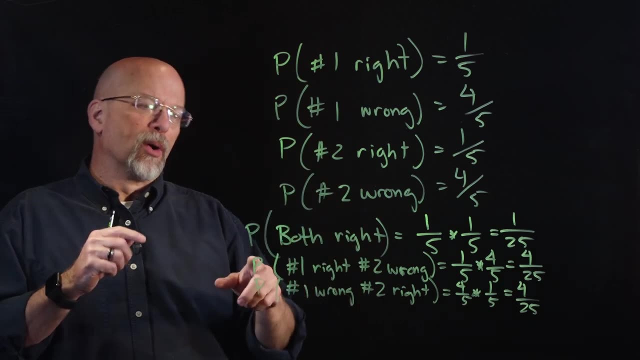 Now, what we're saying here at this point is that there are nine Remember, so we've got, or Remember there was the or option also, So I could look at getting both right, or number one right and number two wrong, or number one wrong and number two right. 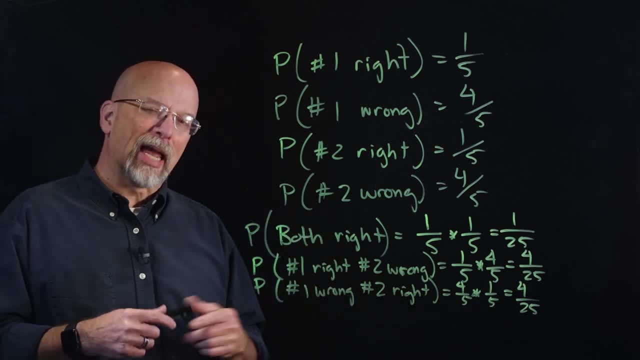 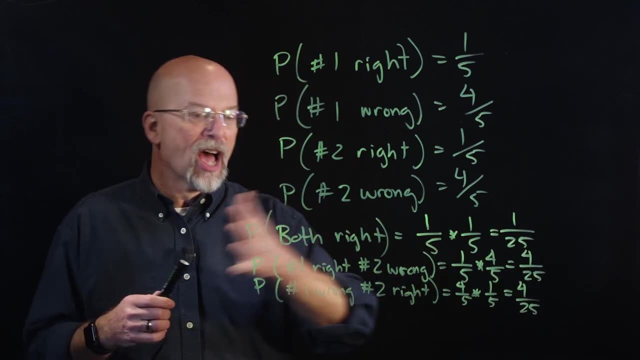 The ors. in that case, we did the additive rule whenever it came to probability, And so we were looking at one plus four plus four or nine-twenty-fifths of one of these, any one of those three cases happening. What is left? 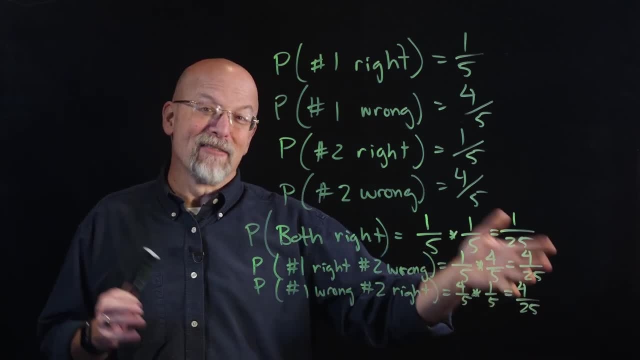 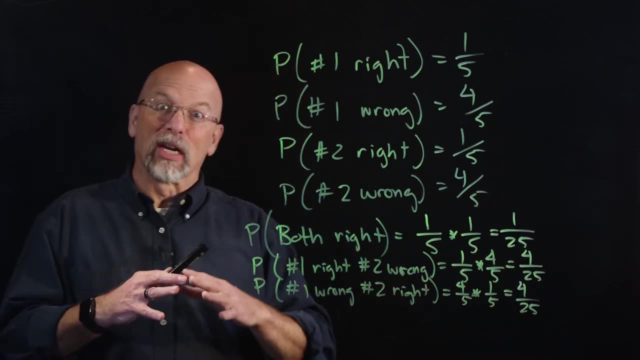 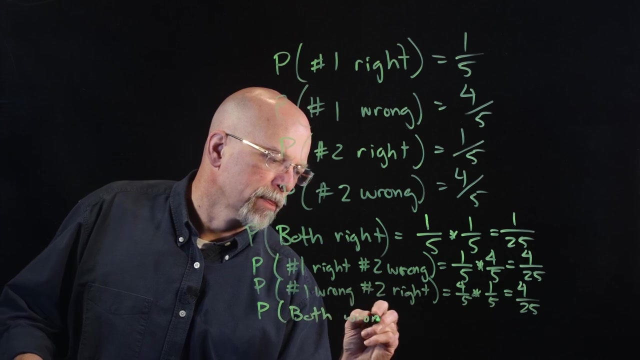 Well, what's left is 25 minus nine. That gives us 16.. Right, So there's actually 16 out of 25 that we're going to get both of them wrong. Does the math work out? Well, the probability of both wrong is equal to four-fifths times four-fifths. 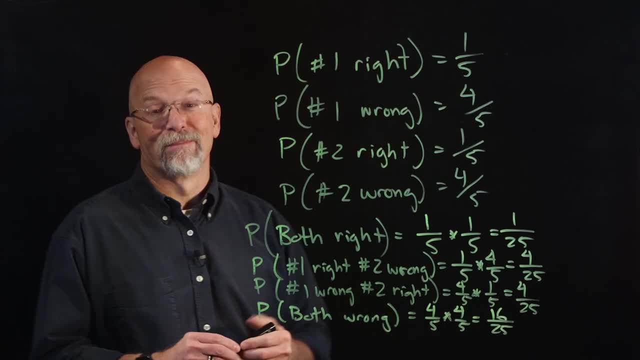 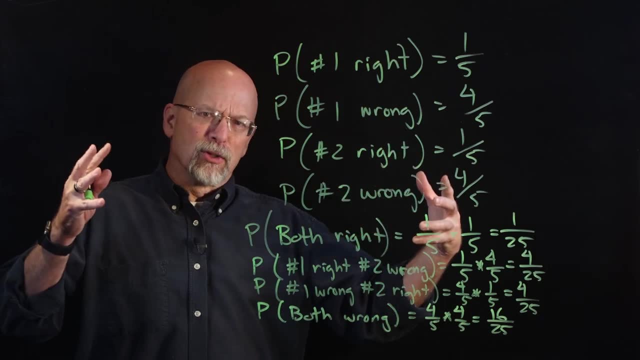 which is equal to 16-twenty-fifths. Yep turned out, the math worked out, So the 25,. in other words, we've got this sample space, the set of all possibilities, That is 25.. There are 25 possible options. 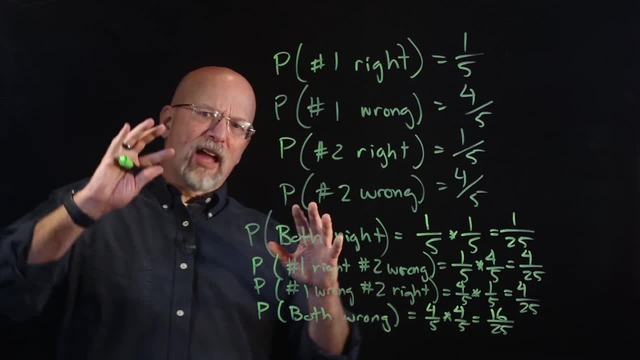 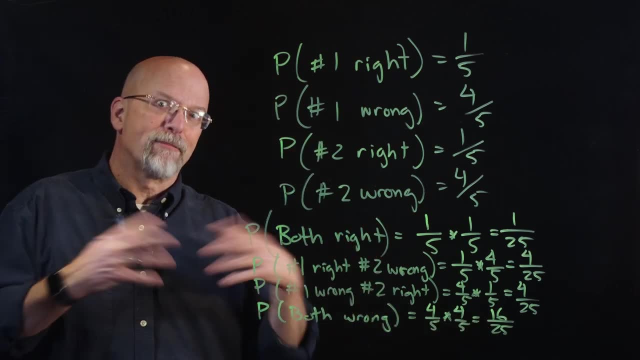 But- and this goes back to the multiplicative rule, Remember, if I've got five options for the first problem and five options for the second problem, five times five gives us a sample space of 25 possible ways that we can answer it. 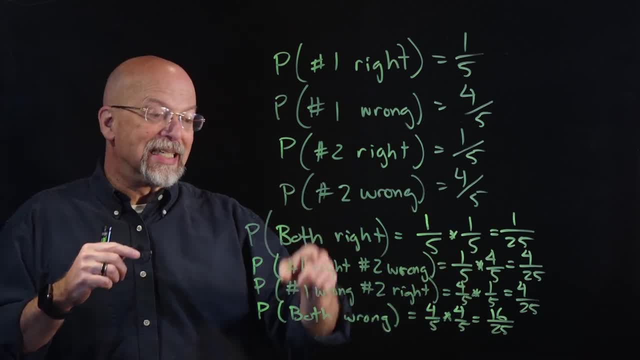 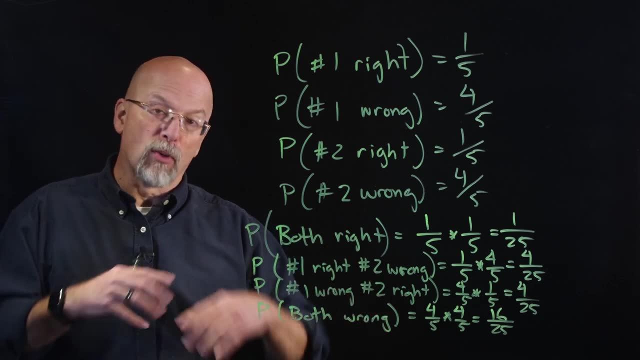 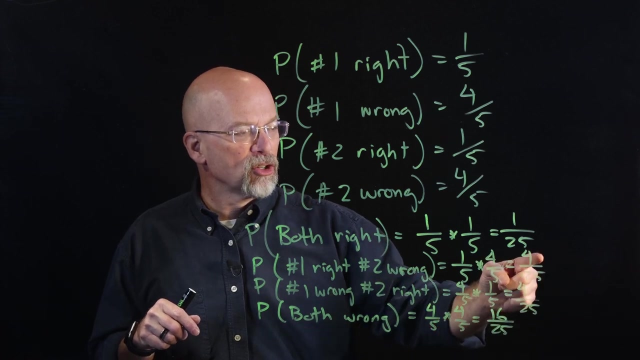 And those 25 ways are separated across the disjoint sets of both right number one right number two wrong number one wrong number two right and both wrong. Those are disjoint events, Event spaces or event sets And since they're disjoint, you can add these numerators together. 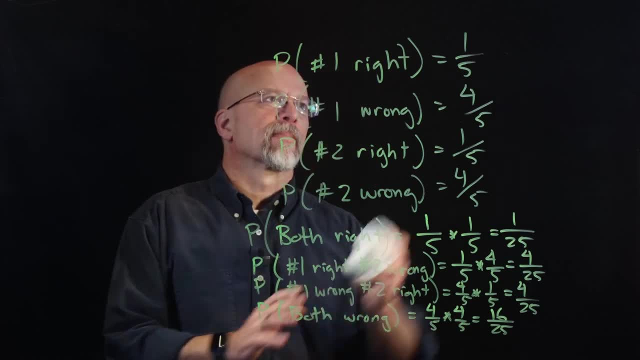 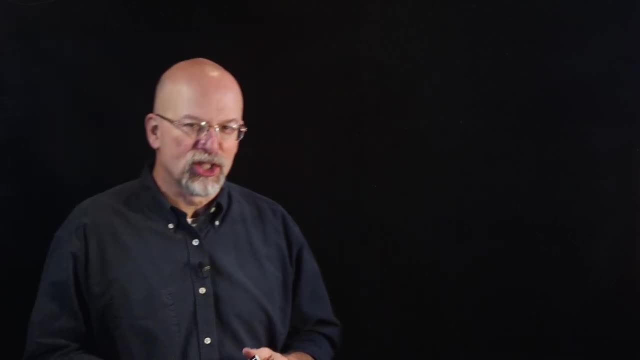 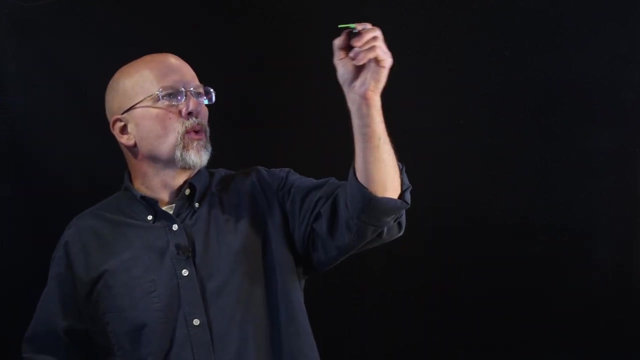 and you should be able to get 25.. Let's make things a little bit more complicated. Maybe we have a four-question test Now. four questions means that let's say that a C is passing, So we're looking for 70% or better. 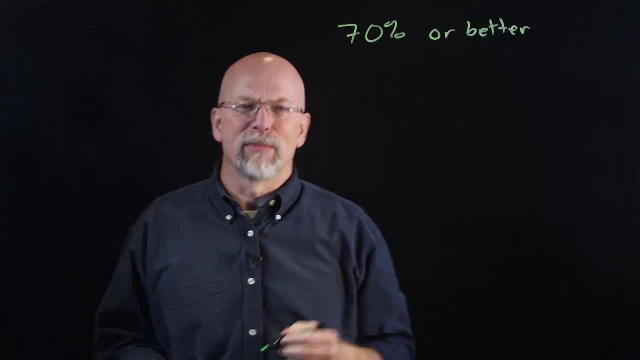 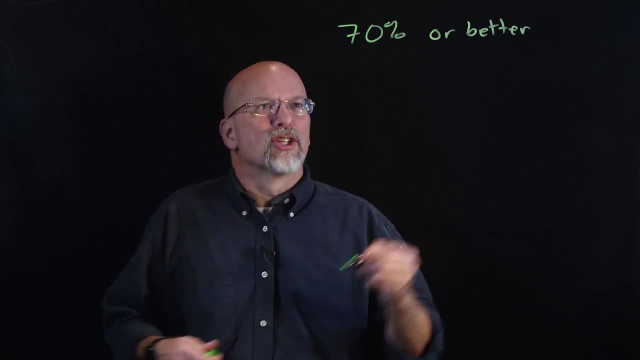 Now the problem is is that you can't get 75%. Excuse me, you can't get 70% with four questions. It's 75%, Three out of four, right? So what we're looking for is at least three correct answers. 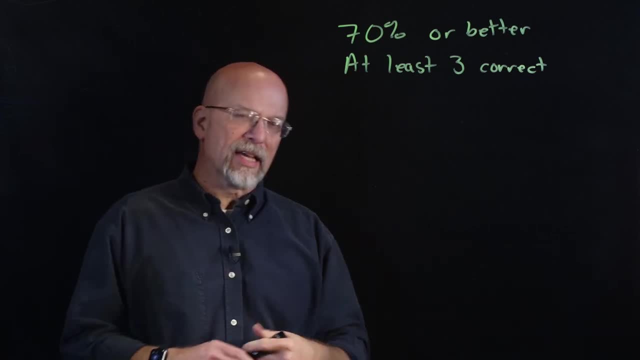 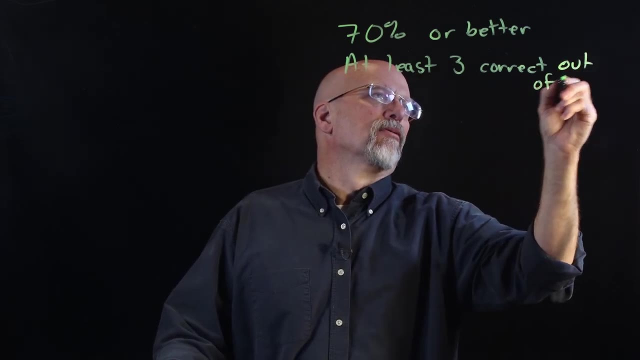 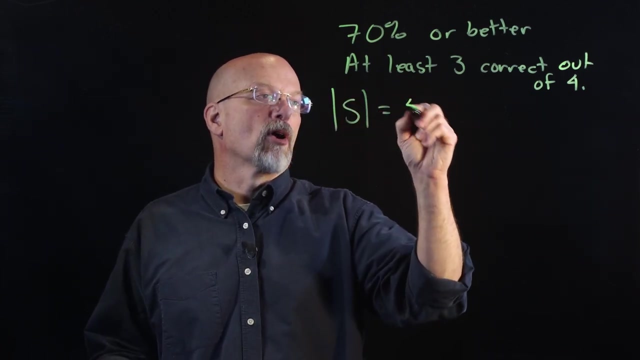 What are our chances if I'm just randomly guessing across four questions? what are our chances that I get at least three correct out of four? Now let's begin with the size of our sample space, the cardinality. Remember, there are five options and there are four questions. 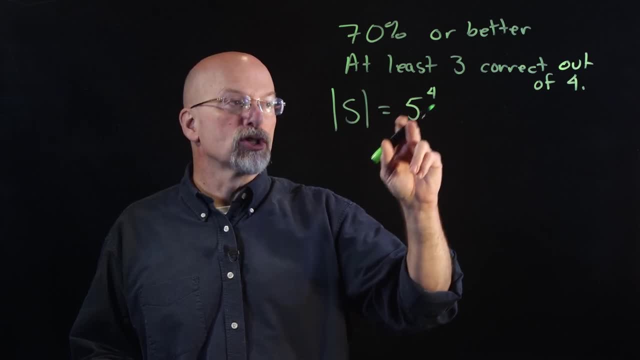 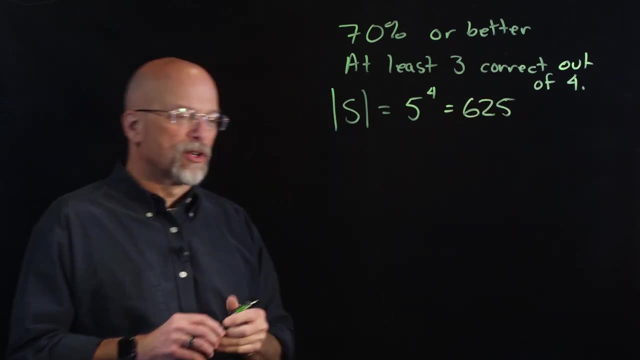 So five options for four questions. So this is really. you're choosing one out of five four times, And this gives us 625, the cardinality of our sample space. Now let's talk about the different ways that we can do things. 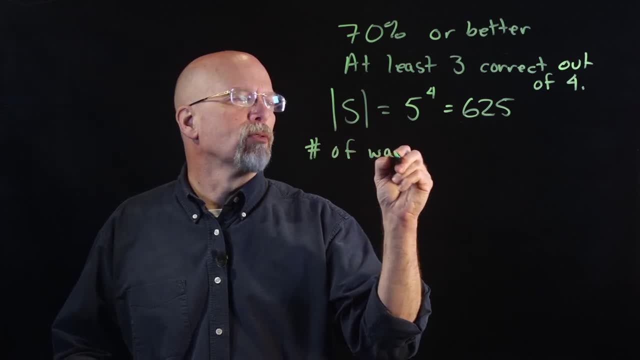 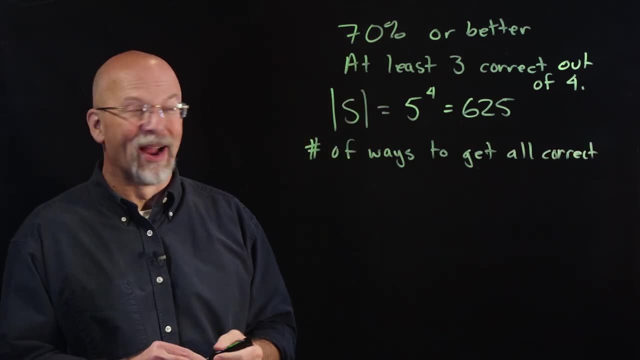 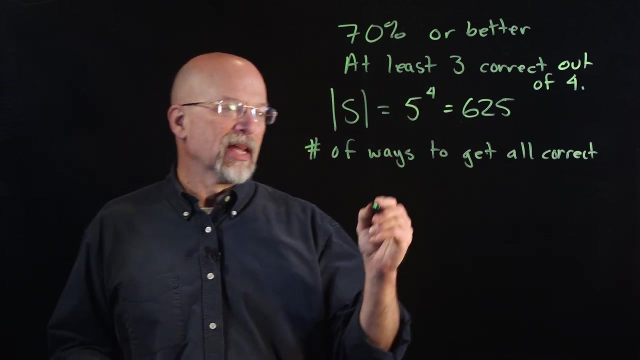 For example, how many ways, so the number of ways to get all correct. Well, there's pretty much one way, right. I have to choose the right one out of each one of those four questions. So what I'm looking at here is the number of ways. 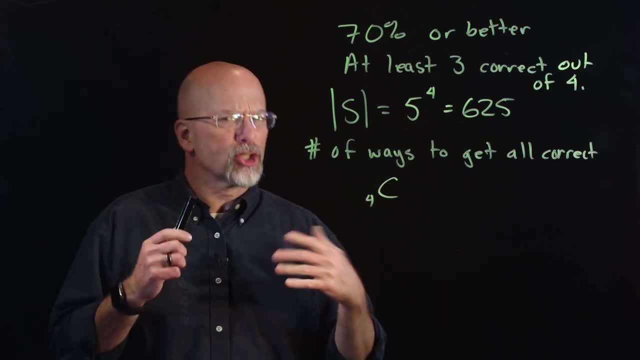 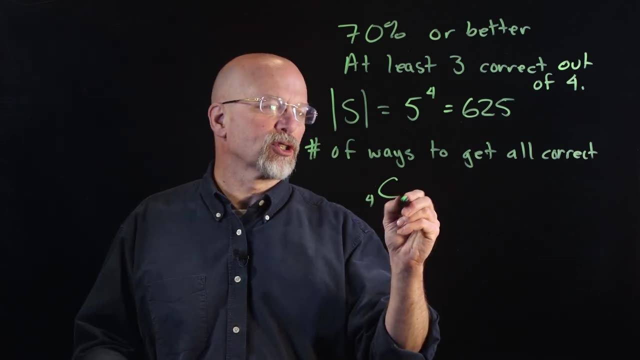 And I've got four questions And what I'm going to do is I'm going to choose which ones I'm going to get wrong. Well, the problem is is that I'm not going to get any of them wrong. So I've got four, choose zero. 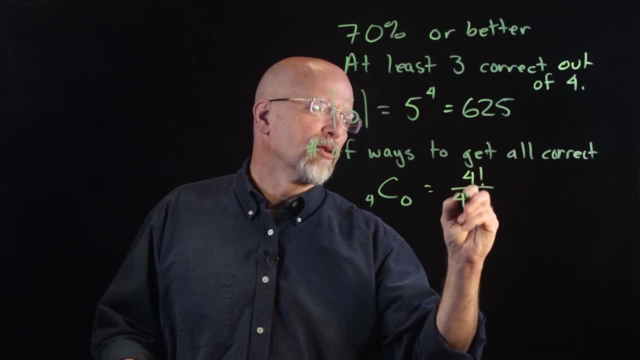 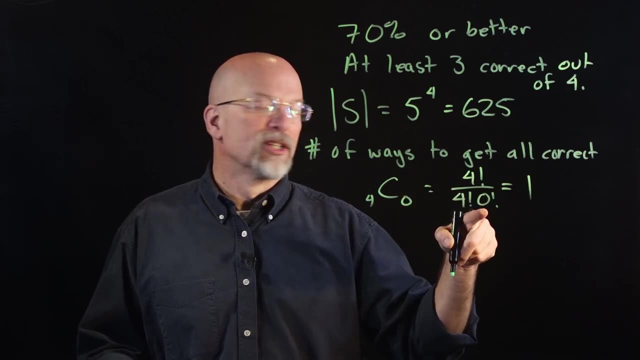 What is four? choose zero. Well, that's four factorial over four factorial times zero factorial, And that's basically four. That's basically equal to one. Four factorial divided by four factorial, that's one. Zero factorial is one also, So this turns out to just be equal to one. 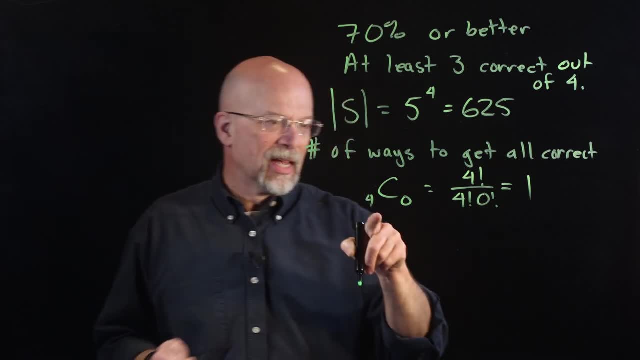 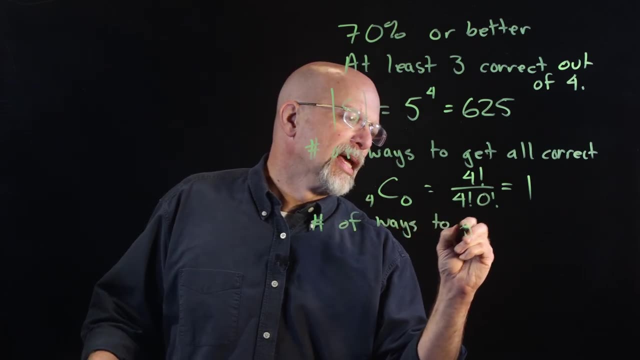 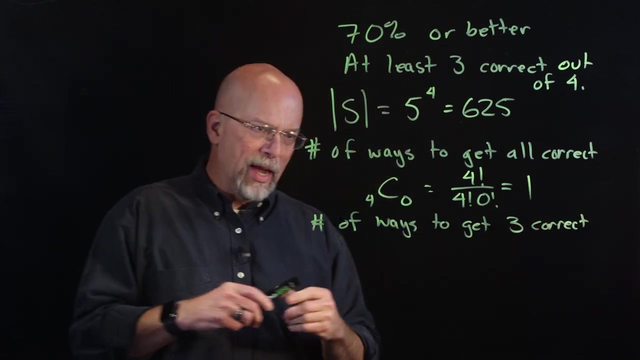 And I have one way to get all of them correct. In other words, I'm choosing to get zero wrong, But what about the number of ways to get three correct out of the four? And so, and we can do this one of two ways. 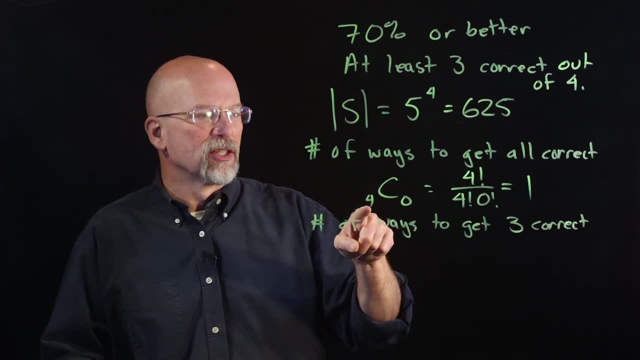 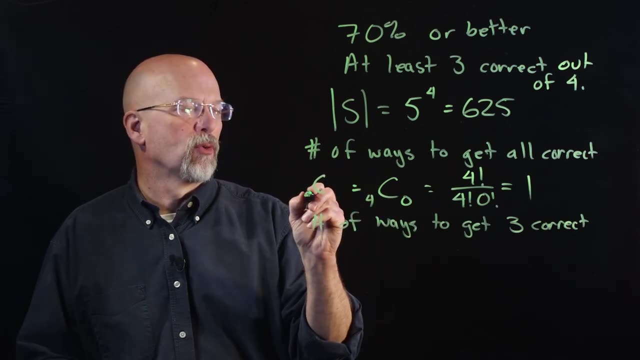 And I said this one way. I said this as four choose four, In other words, I'm choosing which ones I'm getting correct. So this should also equal four choose four. All right, But what about the number of ways to get three correct? 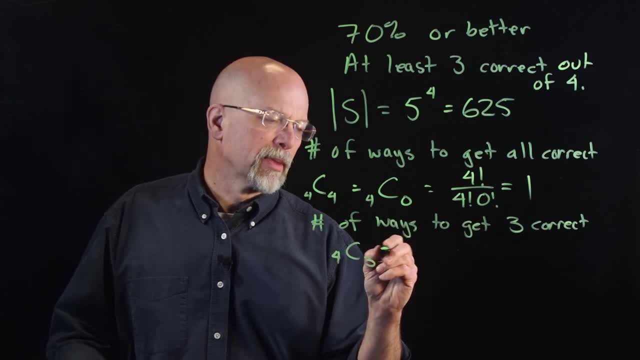 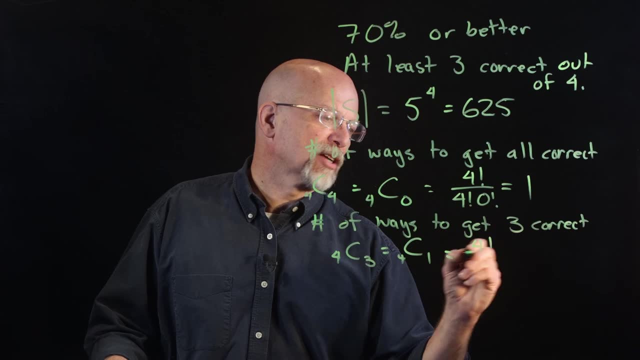 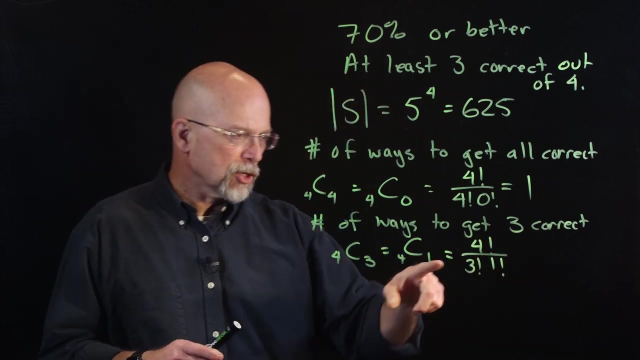 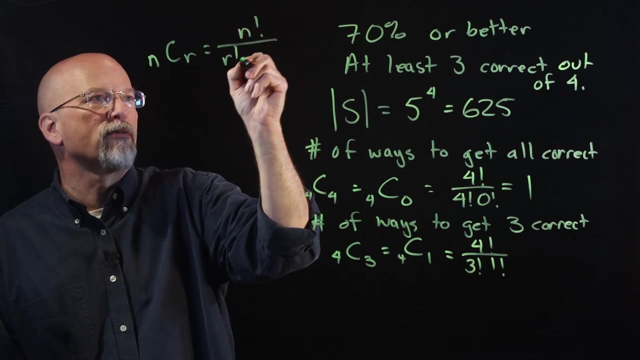 That would be four choose three, Or equal to four choose one, to get incorrect. So these two should be equal And what you get is four factorial over three factorial times one factorial. All right, So remember this expression: The n choose r is equal to n factorial divided by r factorial. 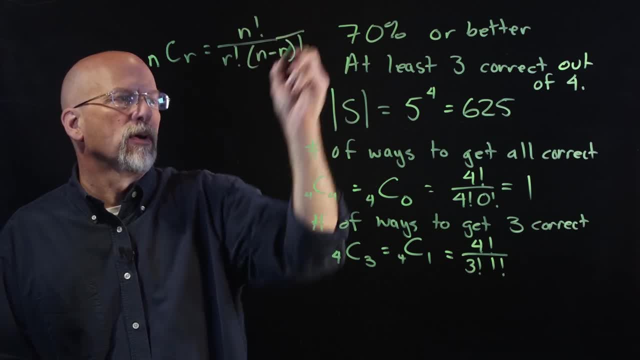 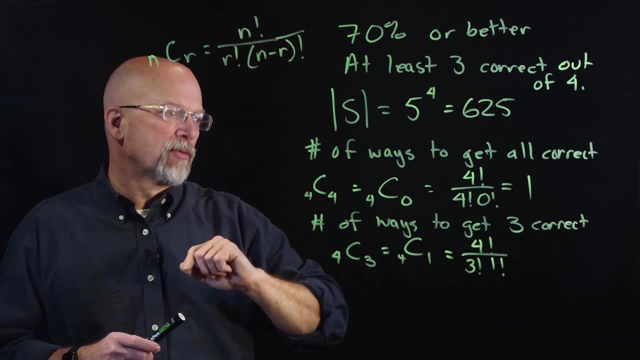 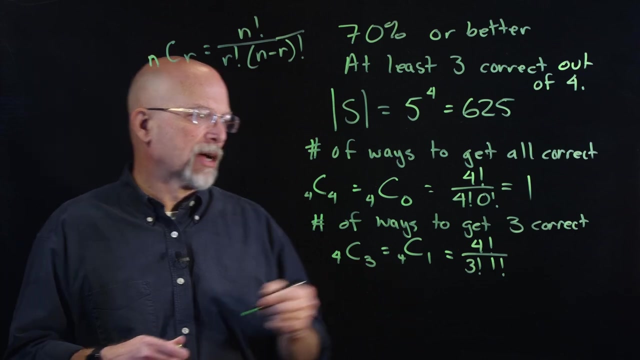 And also divided by n minus r factorial. And so whenever we're looking at four, choose three, that'd be four factorial divided by three factorial times one factorial. Or four, choose one, that would be four factorial divided by one factorial times three factorial. 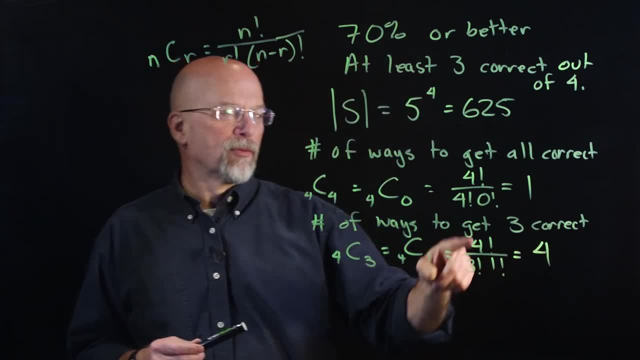 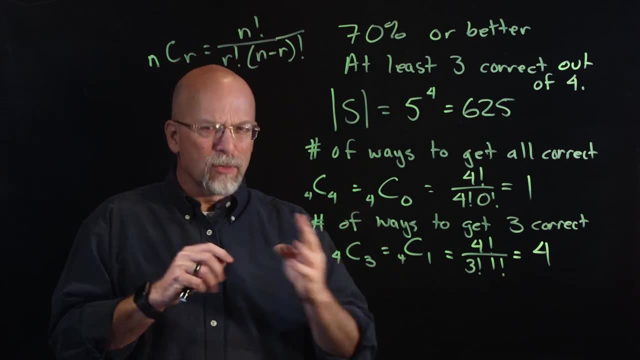 So anyway, that gives us Three factorial divides into four factorial and you get four left over. So there are four ways to get three correct. And that makes sense, because if I've got four questions that wrong, one can be in one of four places. 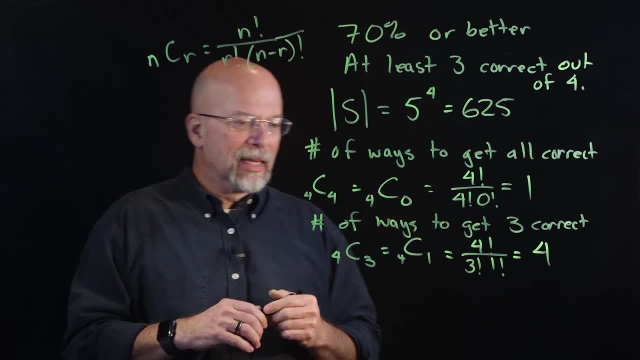 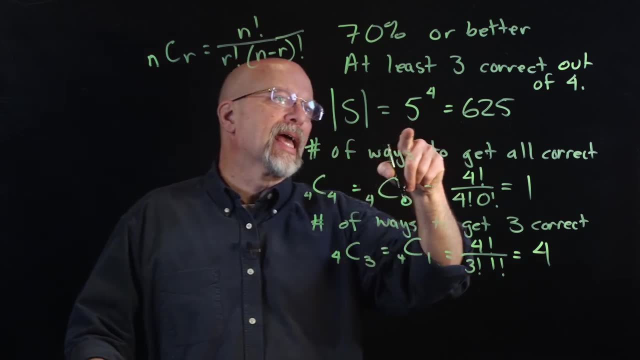 Now the question is: is what is the probability now for each one of these? you know each one of these ways. Well, first of all, the probability to get one, the sample size of one. there's one option out of the 624.. 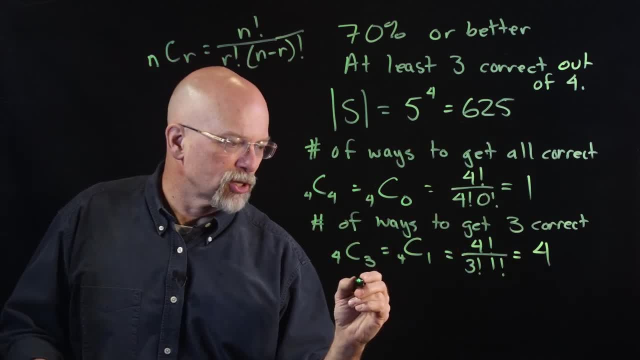 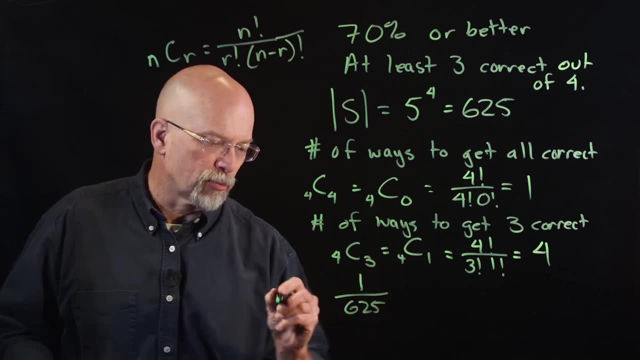 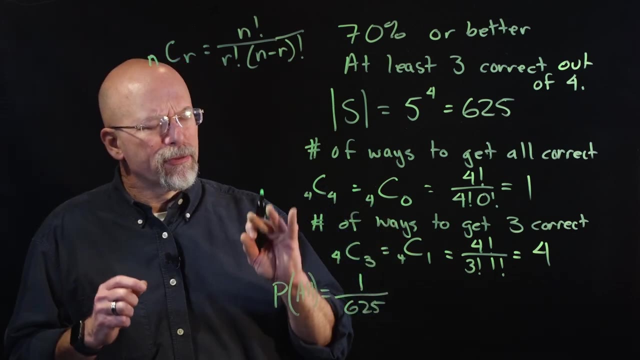 That's 625, in order to get them. you know it right. So that is one over 625.. And so this right here is the probability of getting all of them correct. Right Now, what is the probability of three out of four? 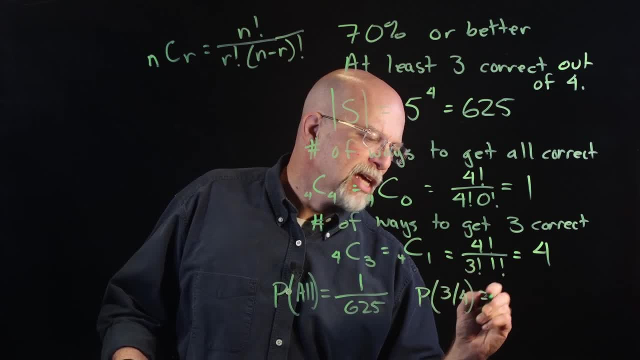 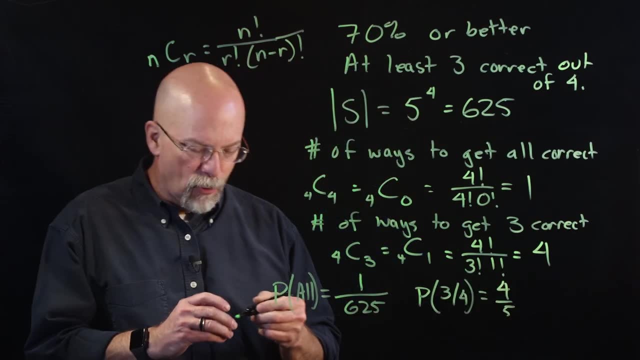 Well, the probability of three out of four is going to be equal to Well, remember to get one incorrect. that is a four out of five. In other words, there are four. there are four ways to get an incorrect answer on one of the questions. 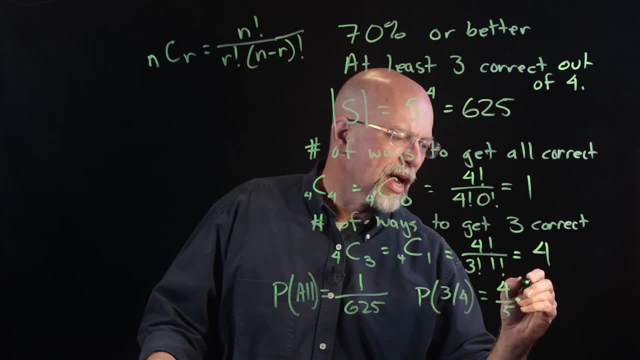 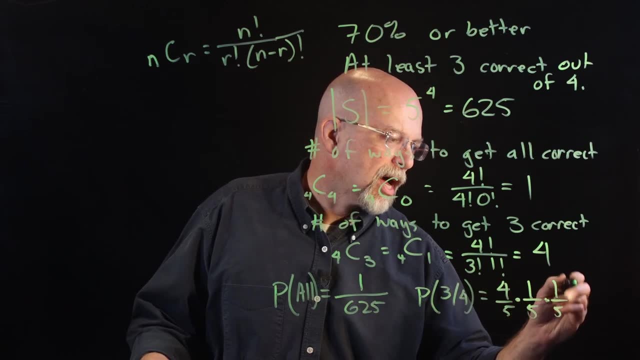 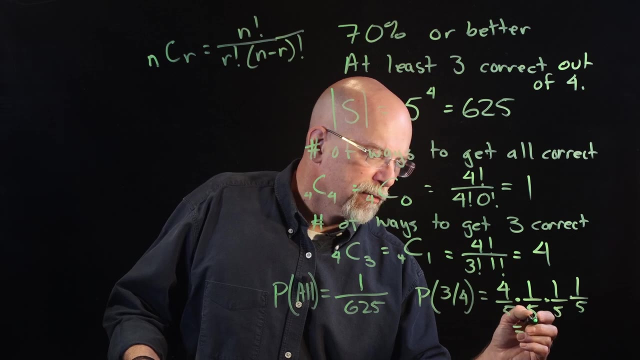 but the other three questions. those have to be all correct. So this has to be times one fifth. There's one way to get the correct answer out of five times one fifth, times one fifth, And that's going to give us a probability to get three out of four correct. of what? 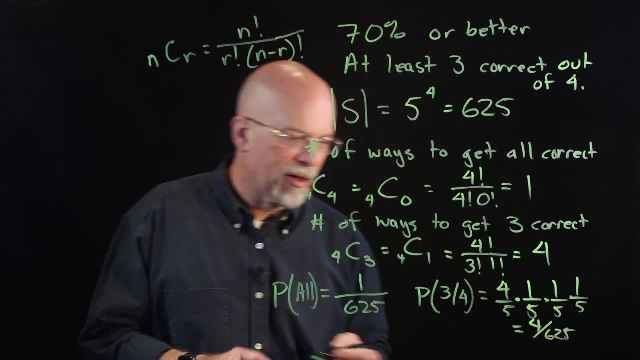 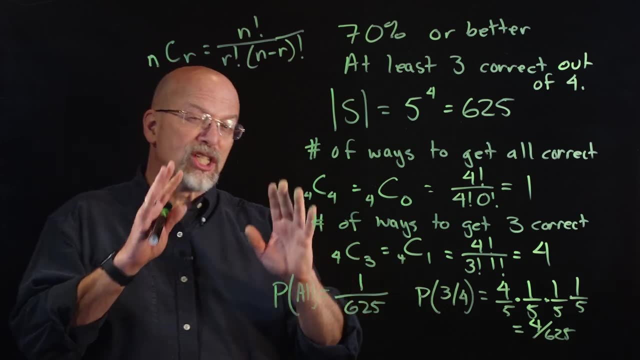 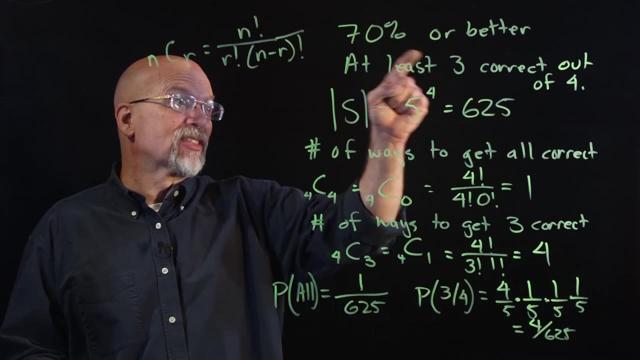 do we have Four divided by 625.. This is the probability that we'll get them all Correct. This is the probability that we'll get three out of four correct for a specific one to be wrong. So what we're looking at is we're going to either get them all in order to get this 75%. 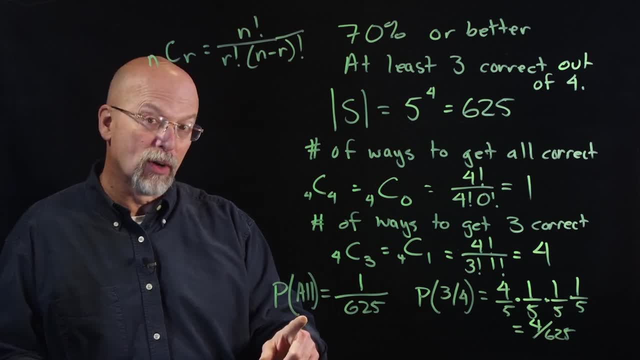 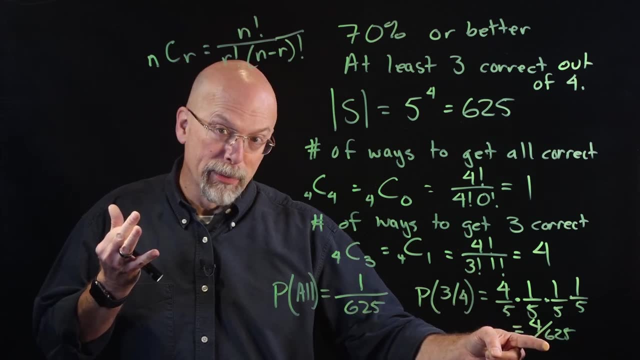 in order to get the grade of 75%, I need to either get them all correct or I need to get the first problem wrong and the other three correct. That's a probability of four. four over 625- or I get the second problem wrong and everything. 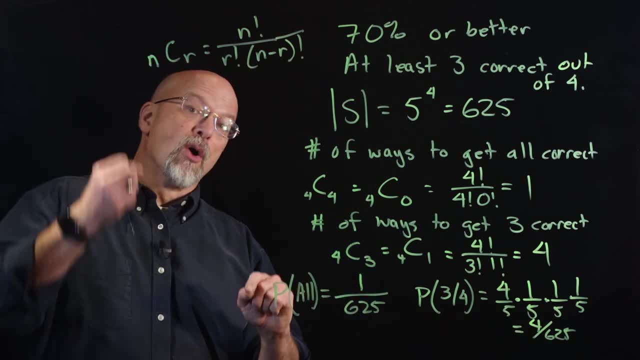 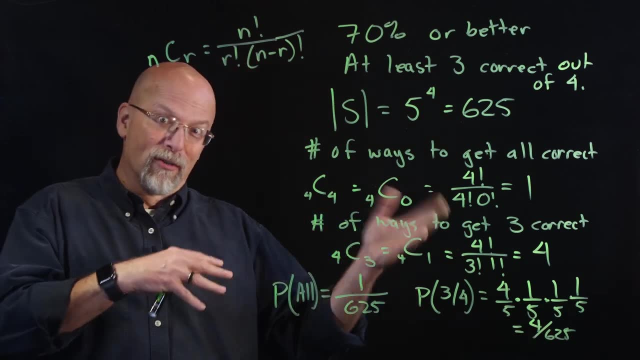 else correct, Which is another probability of four over 625 where I get the third one correct and, excuse me, the third one wrong and everything else correct. There's another one of the four over 625 where I get the last one incorrect and everything else correct. 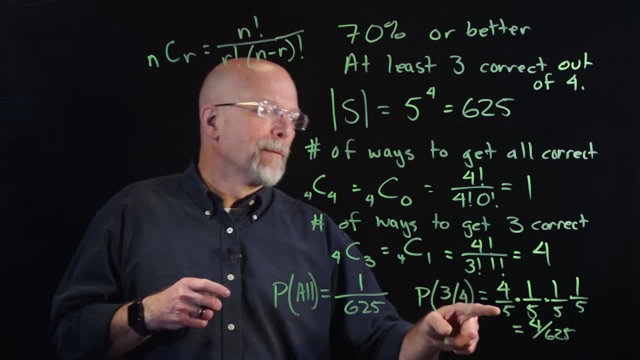 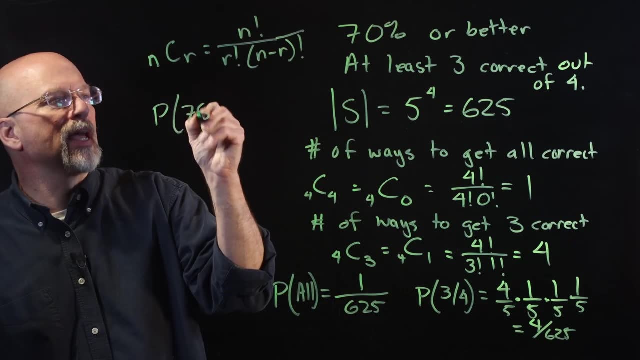 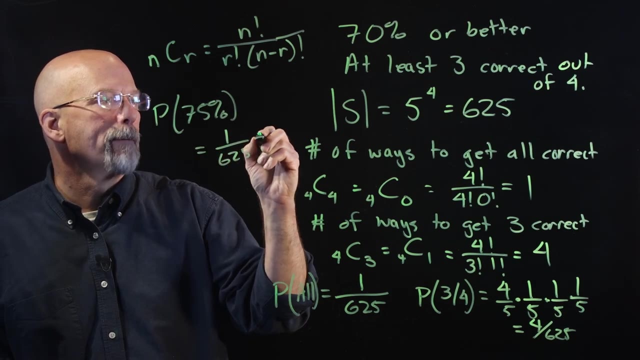 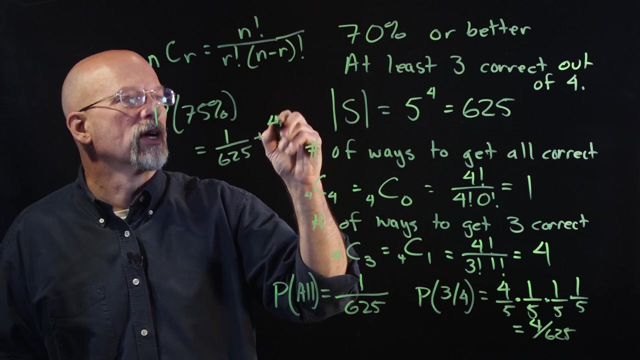 So what I've got is one over 625 plus four times four over 625. So the probability of a grade of 75% or better is equal to one over 625.. over 625 plus the four ways, the four ways, there we are, the four ways that I can get just one. 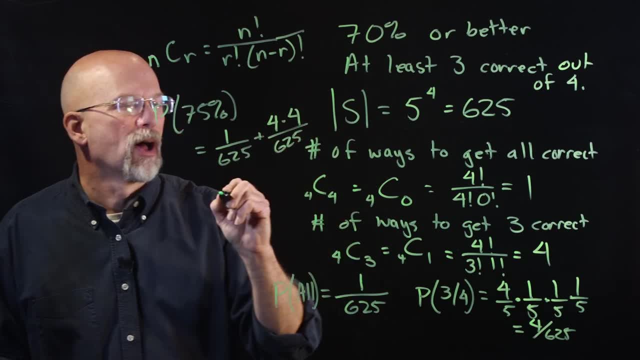 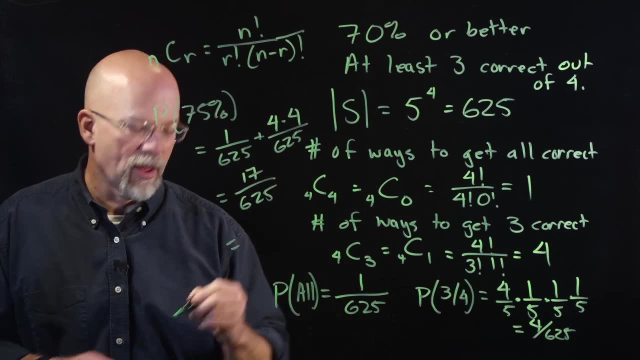 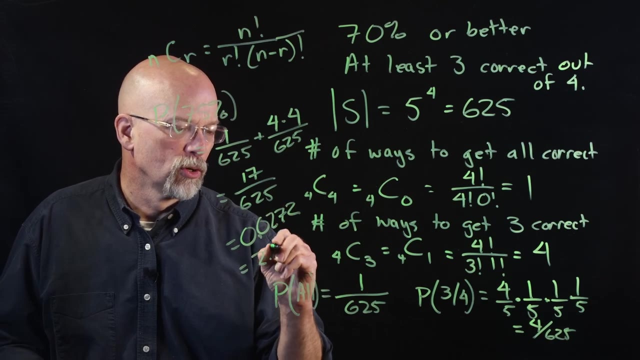 correct. So four times four over 625. And my answer in that case is: four times four is 16.. So we have 17 over 625.. Well, that is equal to what? 0.0272, which is equal to 2.72 percent. 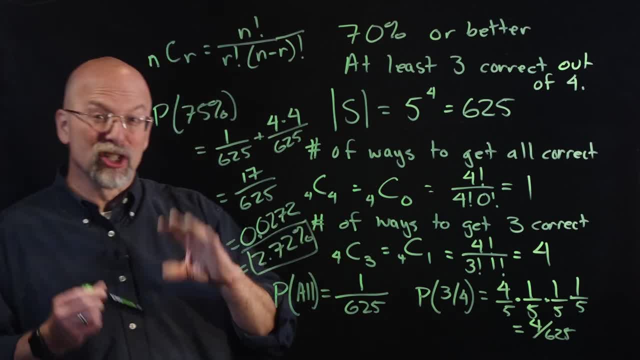 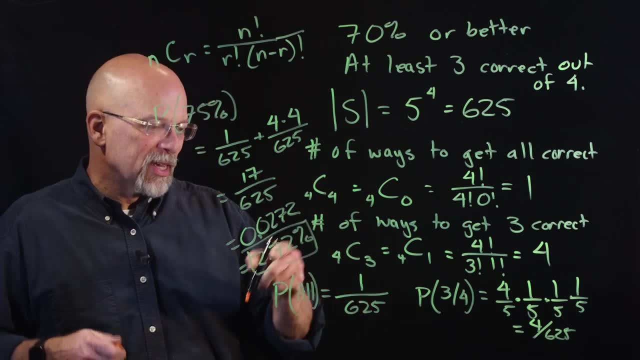 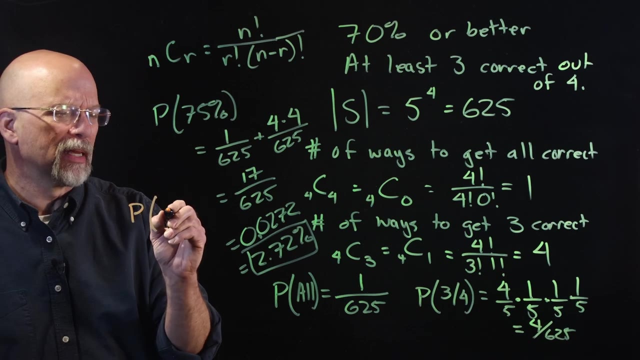 Wow, That's not a very good chance, Just out of four problems, to be able to get a passing grade. 2.72 percent, That means that this 2.72 percent, that's the chance we have to pass. What is the probability that we're going to fail? Well, the probability of less than 75 percent. 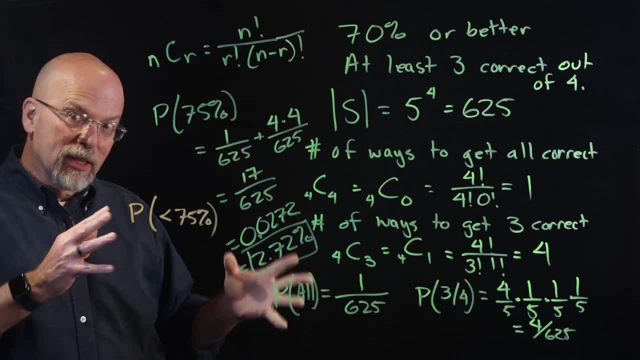 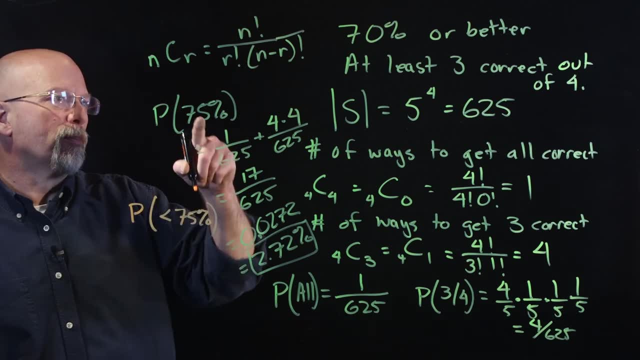 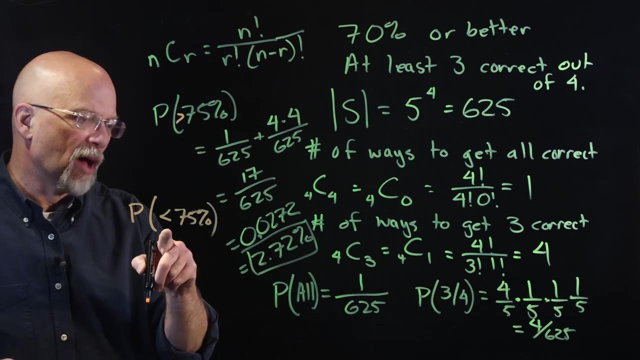 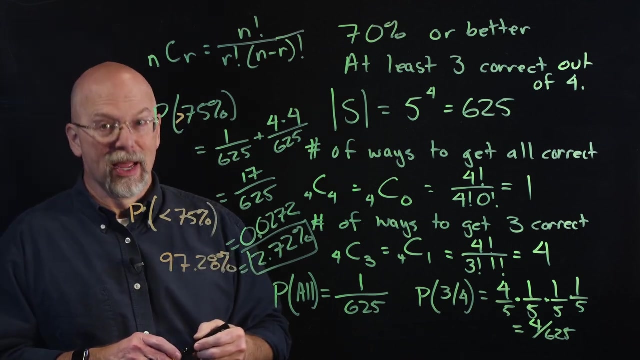 Remember that all the probabilities of disjoint sets that make up an entire sample space they all have to add up to one. So if the probability of greater than 75 percent is 2.72 percent, then that means the probability of less than 75 percent is 97.28 percent. Let me clear this board and we'll see if that's right. 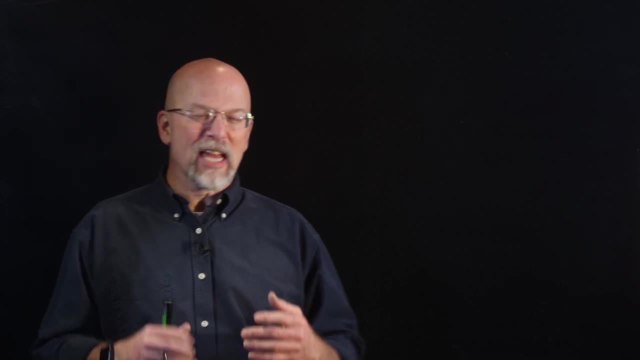 Well, if our probability is only 2.72 percent to get three right or four right on a four problem multiple choice test that has five options, then we're going to fail. So if the probability of less than 75 percent to get three right on a four problem multiple choice test that has five options, 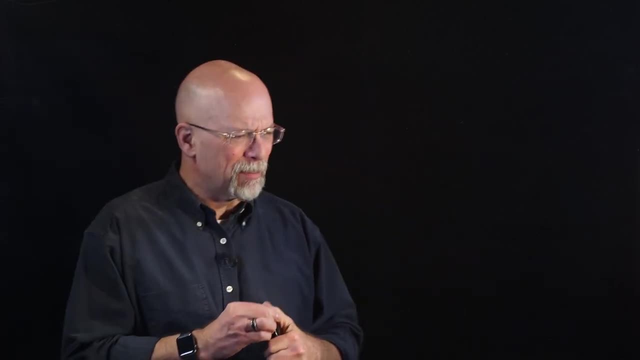 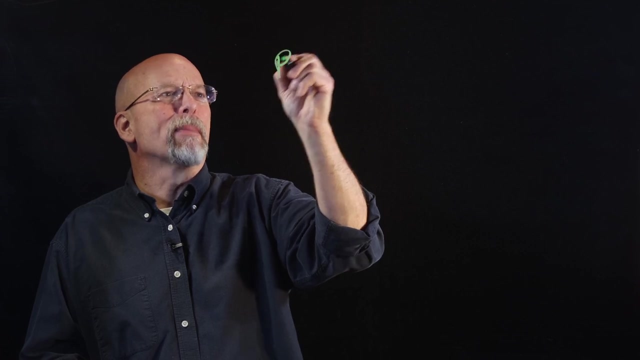 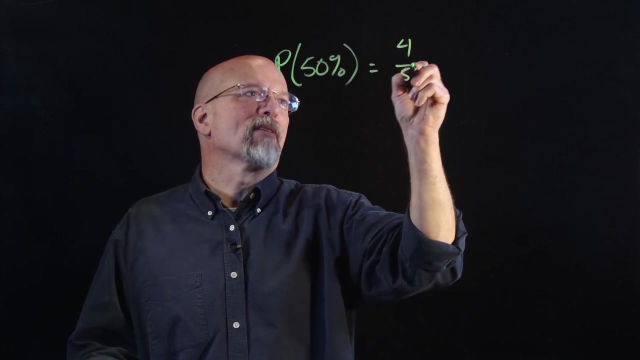 for each problem. that leaves only 97.28 percent. Does that make sense? Well, remember what we're looking at is. well, first of all, let's look at the probability that you got 50 percent right, half of them. Well, if you got half of them right, that means there was a four out of five. 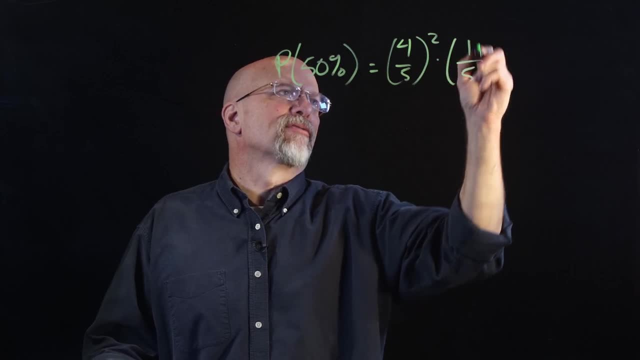 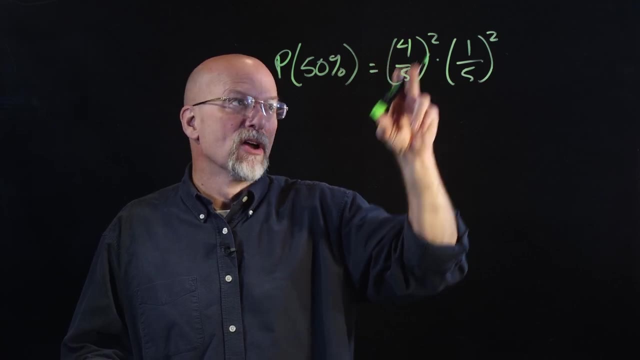 squared for two of them and a one out of five for two of them. In other words, two of them. you got wrong. You picked one of the four wrong ones out of five for two problems and one of them correct out of the five for two of them, And so this gives you what? 16? 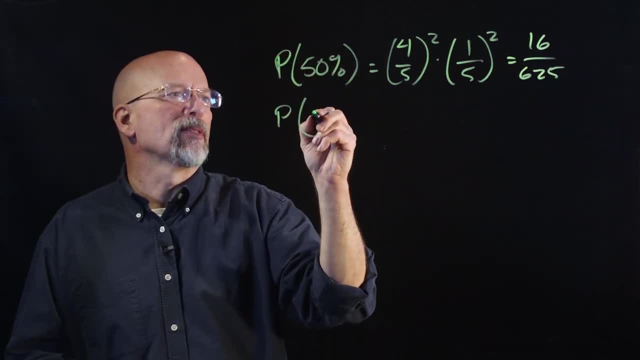 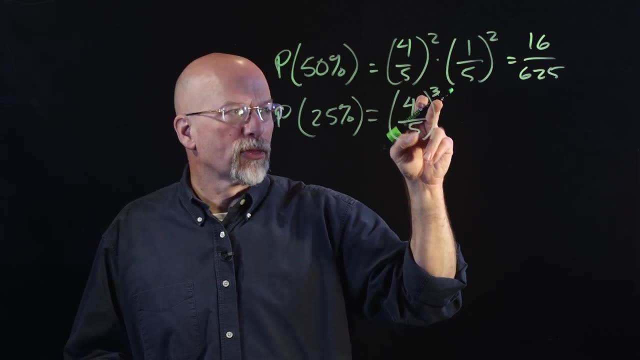 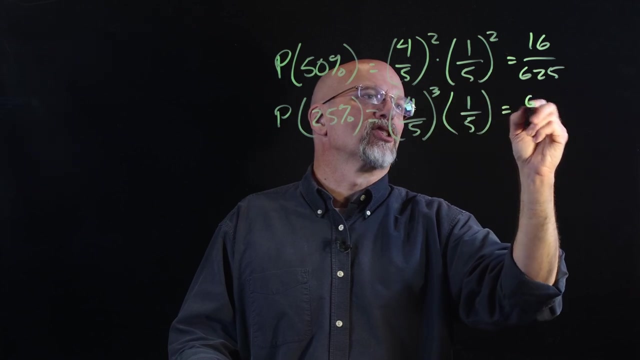 over 625. And then you have the probability that you got only 25% correct And that is going to be four fifths, cubed for the three that you picked wrong times one fifth for the one that you got right, And that's going to give us what? 64 over 625.. And then there's also the probability that 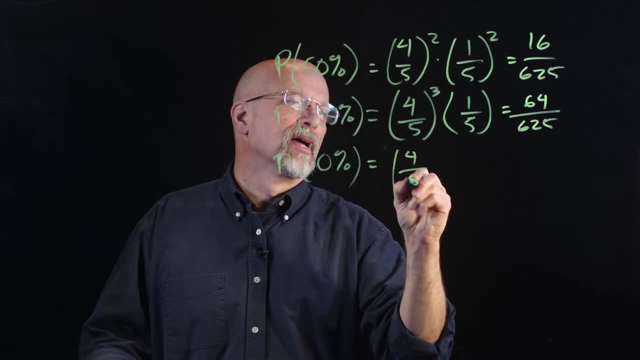 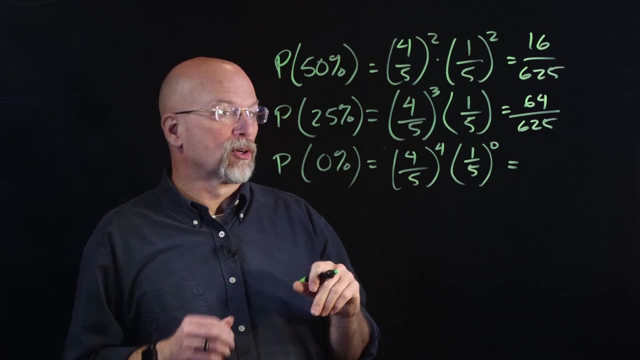 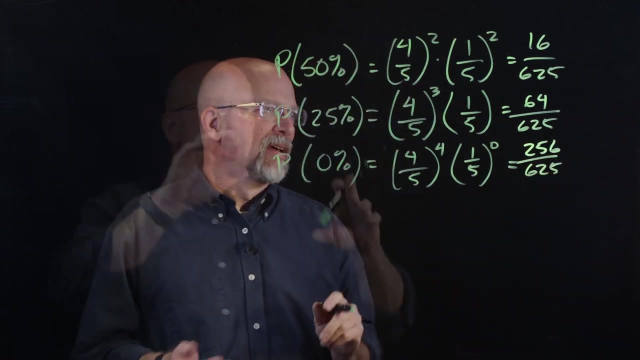 you got none of them correct, And that is four fifths to the fourth times, one fifth to the zero. That's going to be one because you picked zero correct. And so what do we have? 256 over 625.. We still have to figure out the number of ways that we can get just two right and the number. 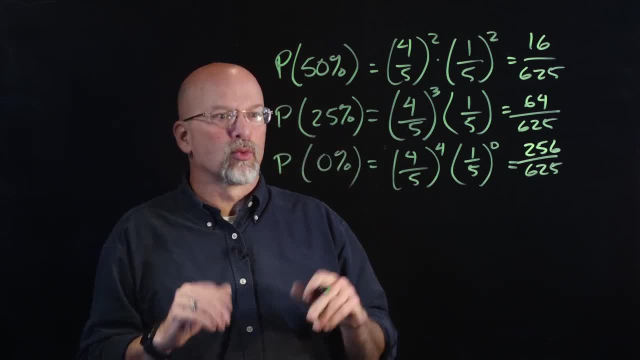 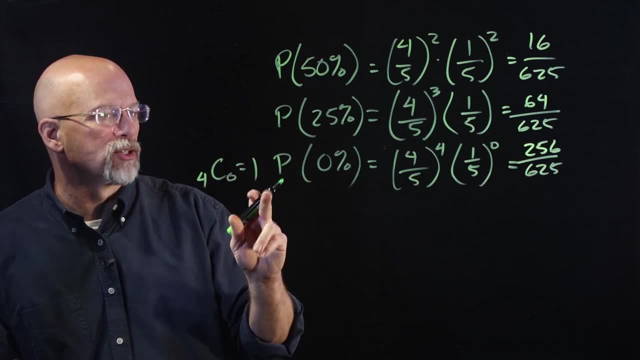 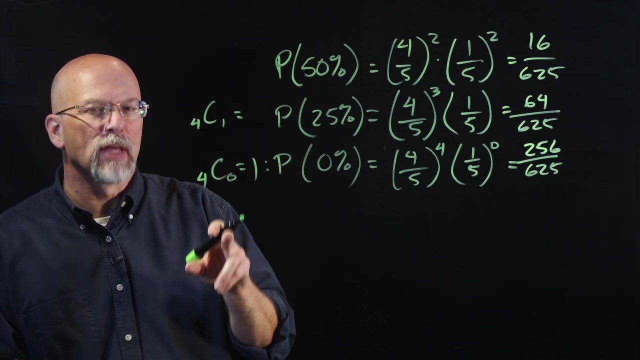 of ways that we can get just one right. There is only one way. you can get none of them right. Remember, we've got four choose zero is equal to one, So there's only one way to do that. But what about four choose one? How many ways were there to do that? Well, if you remember, whenever we looked 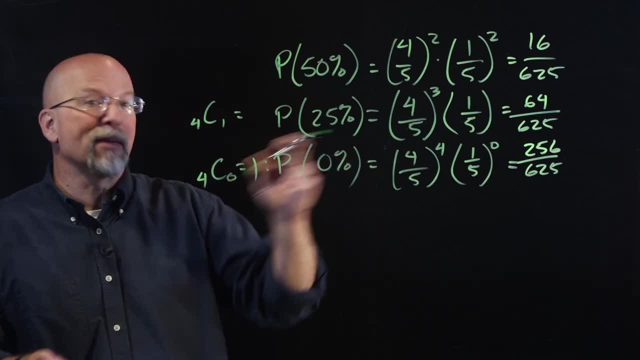 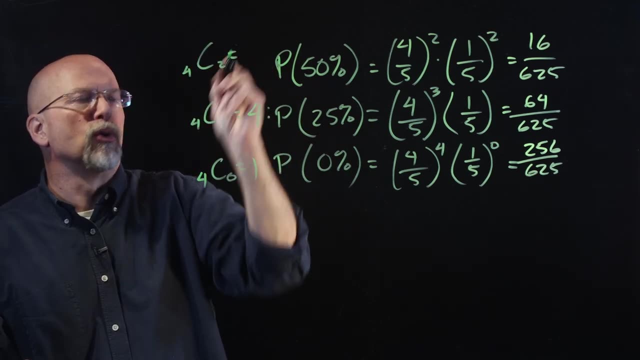 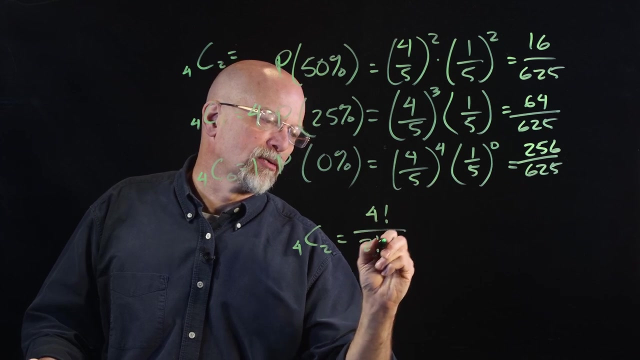 at choosing which one we got wrong. that's the same as choosing which one we got right. So that's equal to four. What about half of them? Four choose two. What does four choose two equal to? Well, four choose two is equal to four. factorial divided by two factorial. 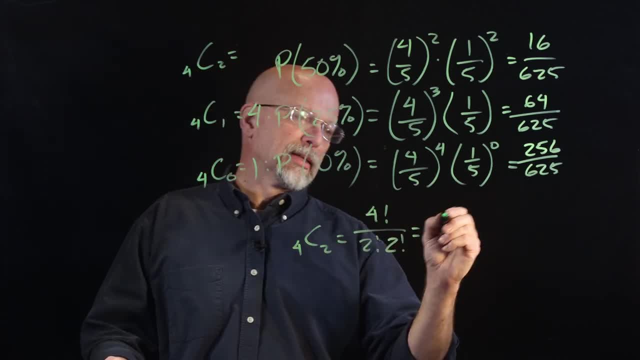 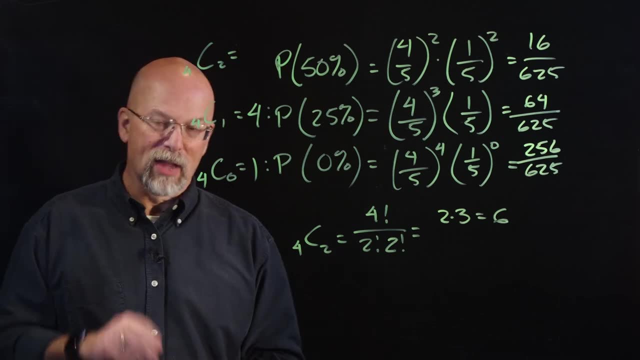 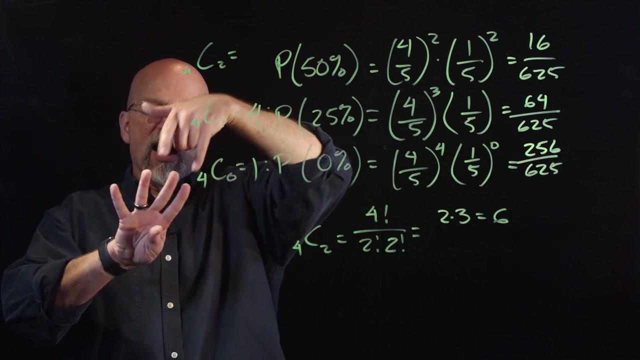 And that'll give us what? Two times three, which is equal to six. So there should be six ways in order to do that. So you've got four of them. I can choose two, I can choose two. I can choose two. There's three ways: Four, five and six. 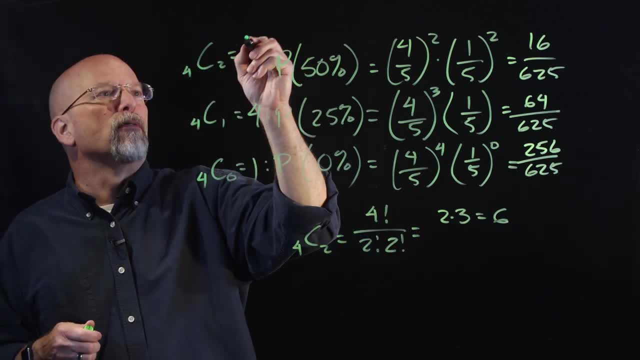 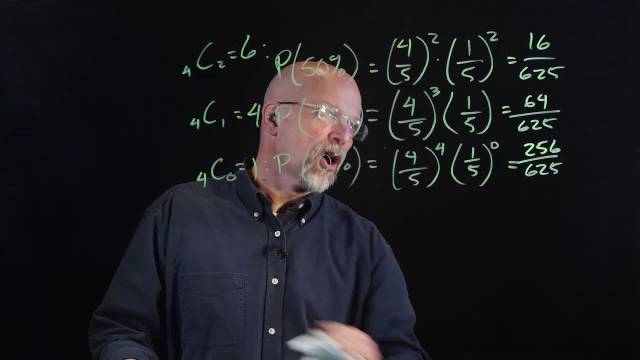 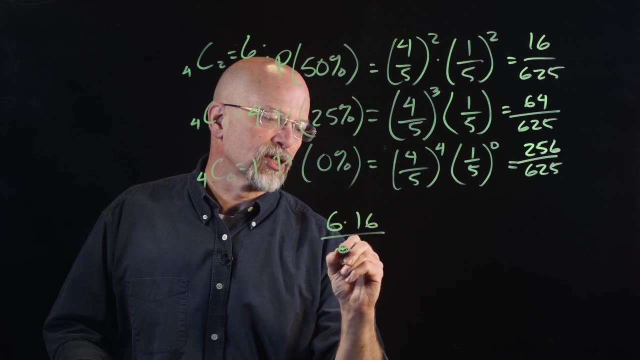 So there are six ways that you can choose two. So four choose two is equal to six. So we come to our expression here. What we've got is 16 625ths added six times, So that becomes six times 16 over 625.. Added to the four ways, we can get 64 over 625.. 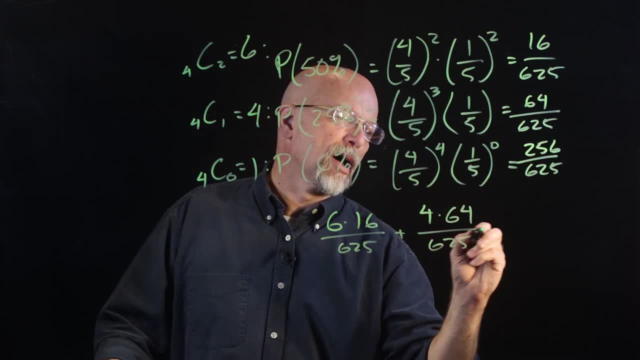 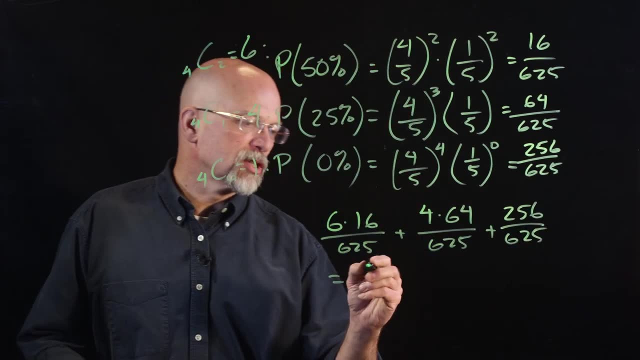 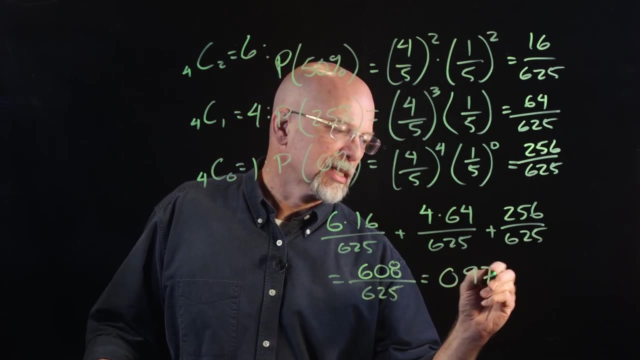 So that's four times 64 over 625.. Plus the one way that we can get 256 over 625.. So this is equal to 608 over 625,, which is equal to 0.95.. So that gives us 9728,. 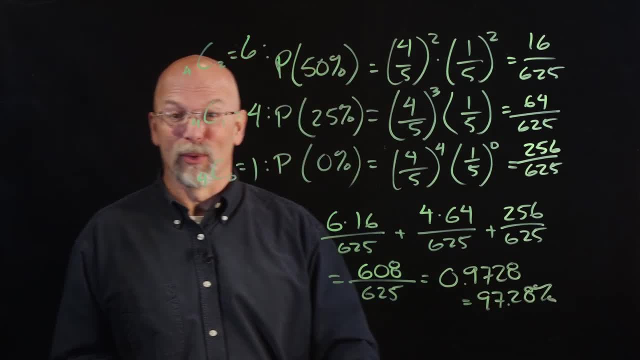 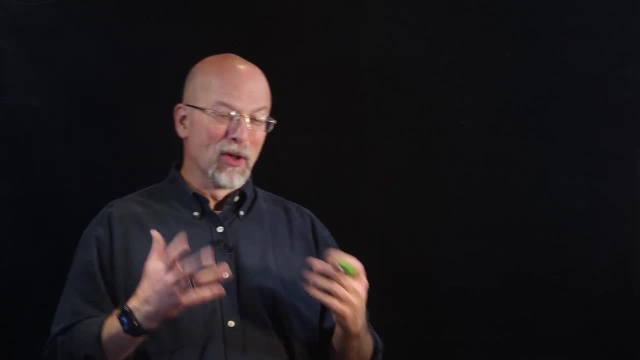 otherwise known as 97.28%. Things don't look good for it. I'm really sorry to keep harping on this idea of a multiple-choice test, But maybe what I'm trying to do is impress upon you the importance of studying for your test. 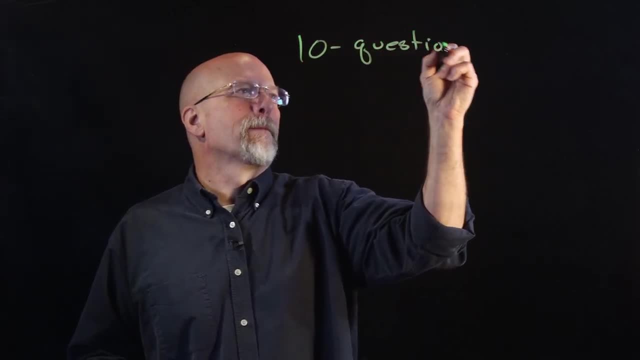 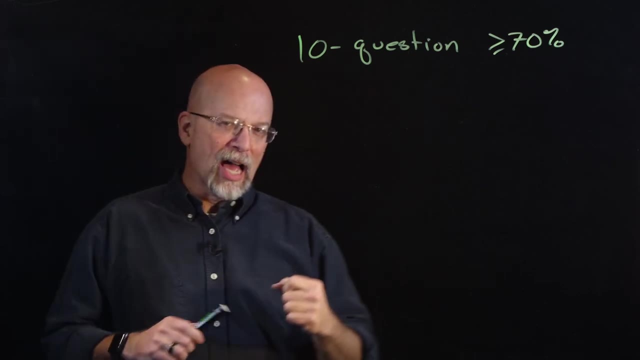 Let's go to ten questions, And in order to pass this, we need to have a better-than or equal to 70 percent, And so that means I can get 7 right, or I can get 8 right, or I can get 9 right, or I can get 10 right. 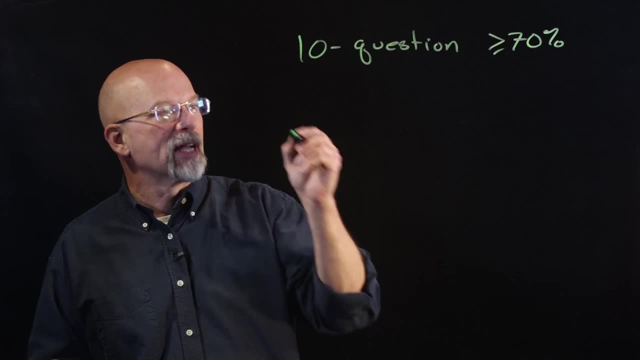 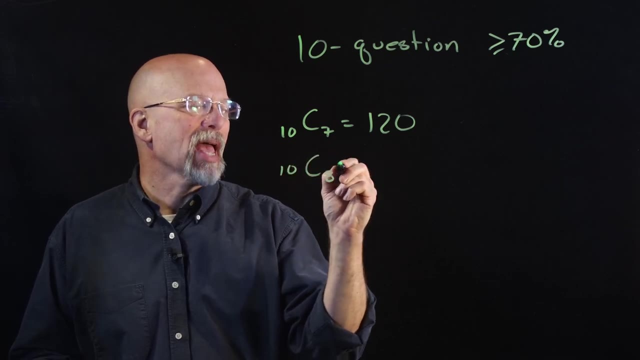 So 7,, 8,, 9, 10.. There are four ways to do that. So we're looking at 10, choose 7,, which is equal to 120.. Trust me, We're looking at 10, choose 8, which is equal to 45.. 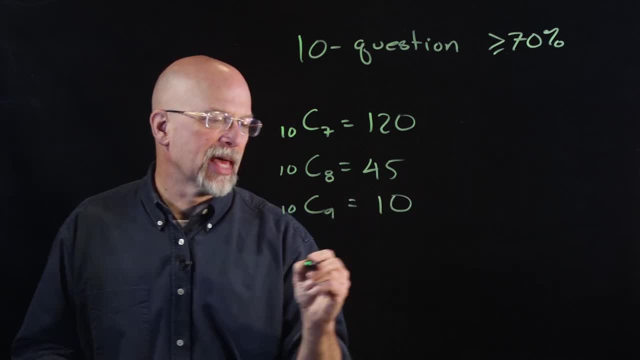 We're looking at 10 choose 9,, which is equal to 10.. Remember, that's the same thing as 10 choose 1, because you're choosing 1 not to be a member, and there are 10 ways to do that. 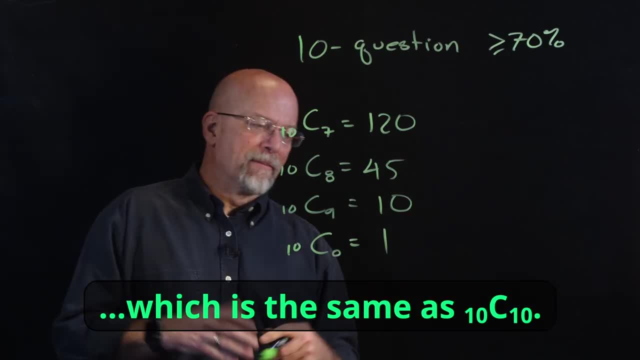 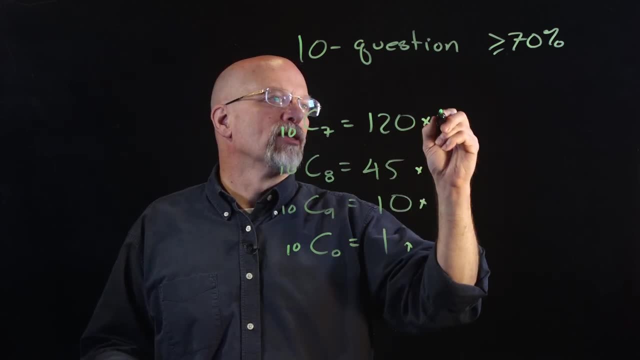 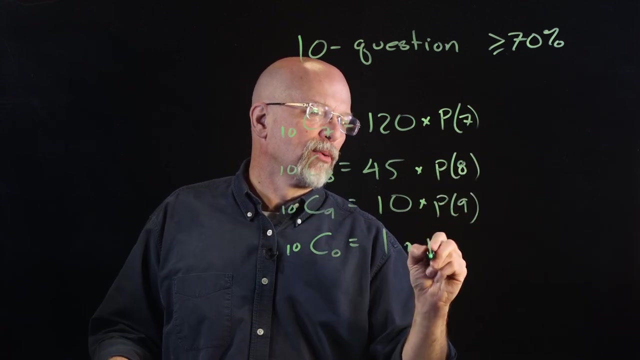 And then 10 choose 0, which is equal to 1.. So there are the number of ways. Now we need to multiply that times the probabilities: The probability for 7 right, the probability for 8 right, the probability for 9 right and the probability for 10 right. 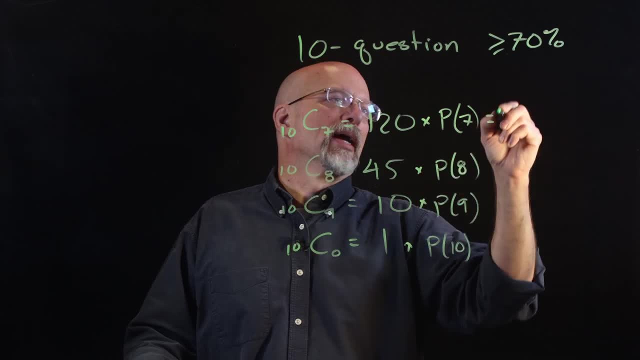 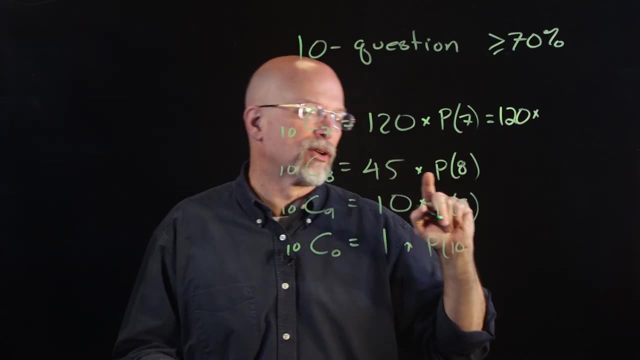 Well, the probability for 7, right? well, that is going to be 120 times, And 120 times, remember, It's the number of ways that we can get 7 right. And so that is equal to 1 fifth to the 7th. 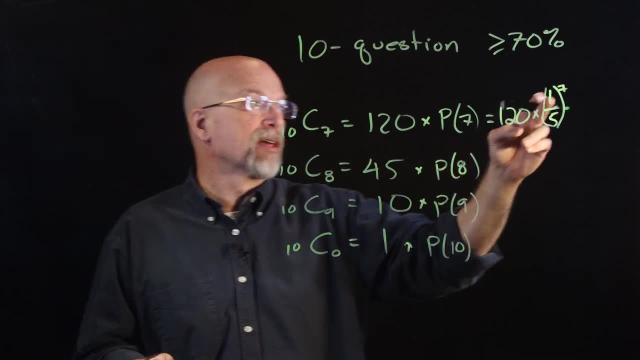 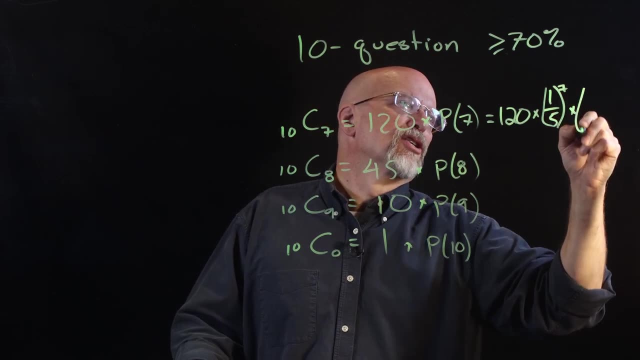 Remember we've got a probability per question of 1 fifth. If I get 7 of those right to get it right. If I get 7 of those right, it's 1 fifth to the 7th, So and then 4 fifths. that's the probability that you're going to get a question wrong. 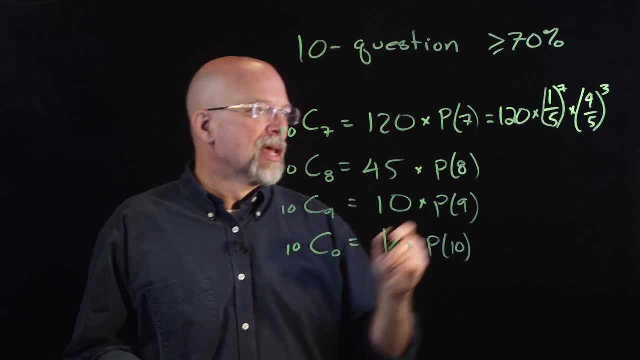 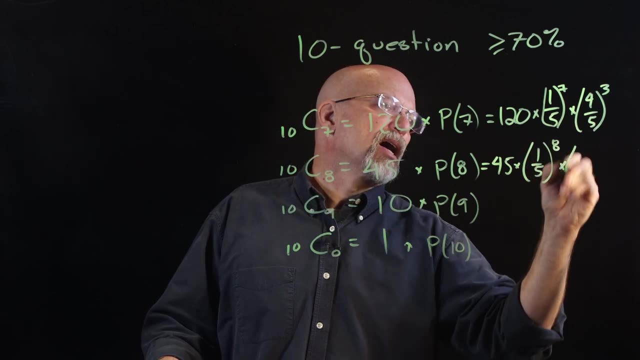 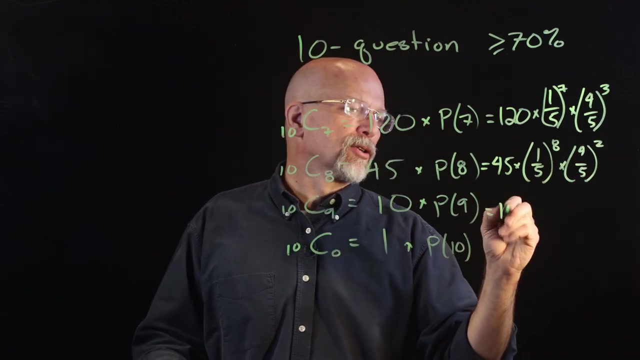 And we need to get 3 of those wrong. right, Then we've got 45.. 5 times 1. fifth to the 8th, times 4 fifths to the squared, And then for 9. right, there are 10 ways to do that. 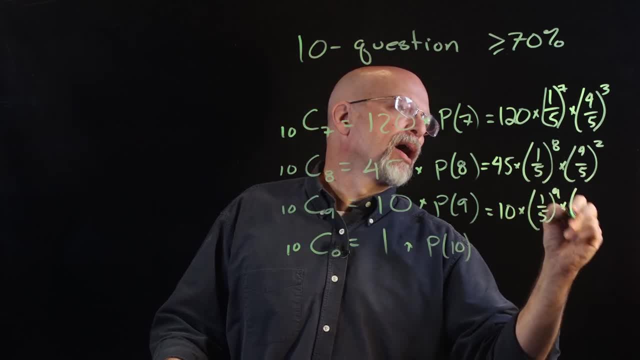 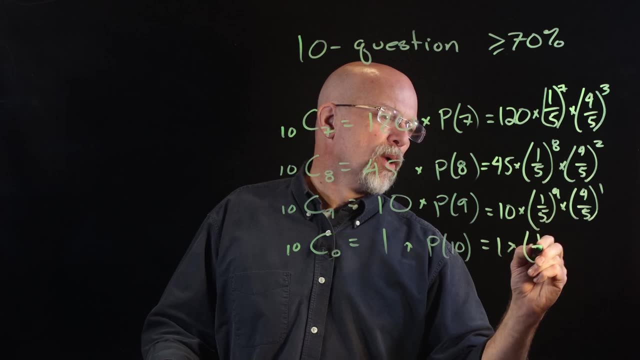 1 fifth to the 9th times 4 fifths to the 1.. And then, last of all, there is one way to get them all right, And that would be 1 fifth to the 10th times 4 over 5.. 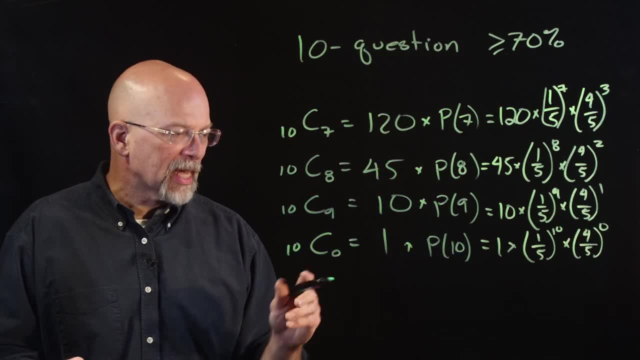 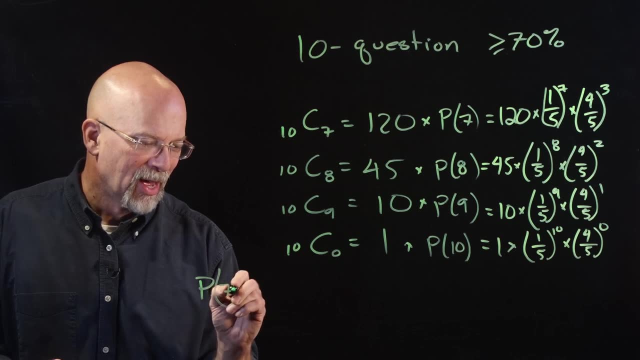 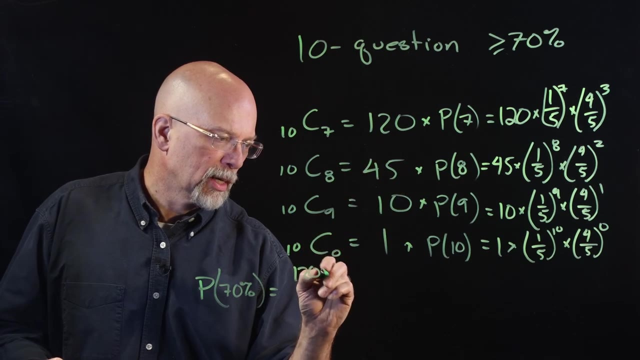 The 0.. Which is going to give us a probability of what do we have. If I'm looking at a probability, I need some space here, don't I A probability of a 70% or better? Then that's going to be our 120 times 64.. 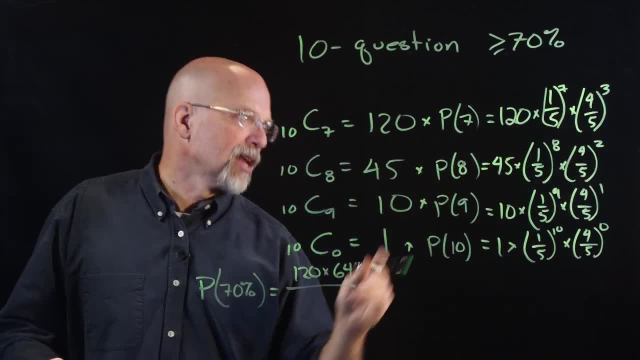 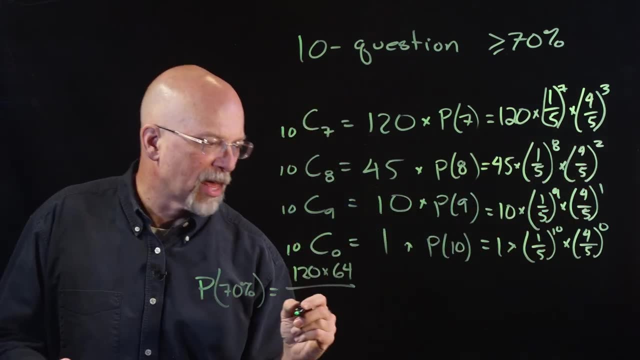 So 4 cubed is 64 divided by, and there's 5 to the 7th times 5 to the 3rd. So this denominator is always going to be 5.. 5 to the 10th. 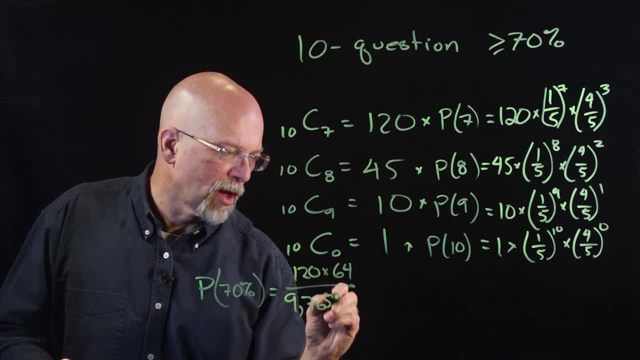 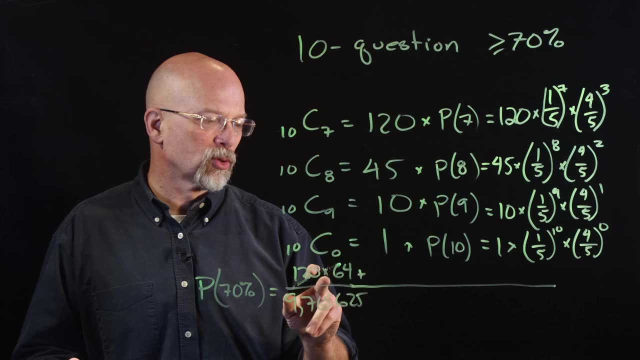 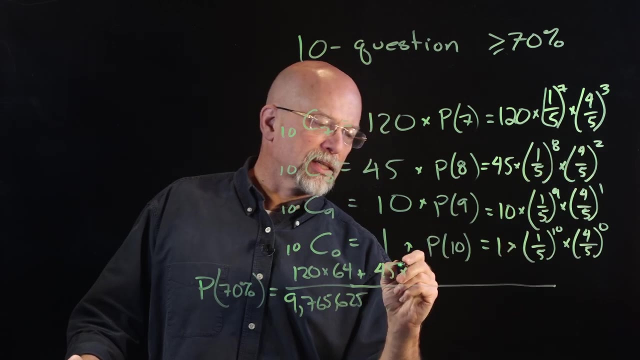 Well, 5 to the 10th is 9,765,625.. And so actually that denominator is going to be the same for all of them. So I'm going to do 120 times 64 plus 45 times, that's 16, right. 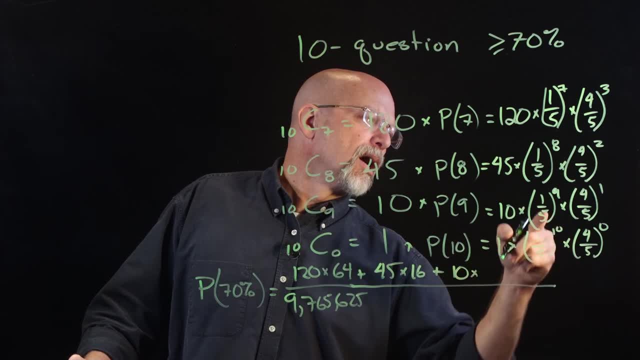 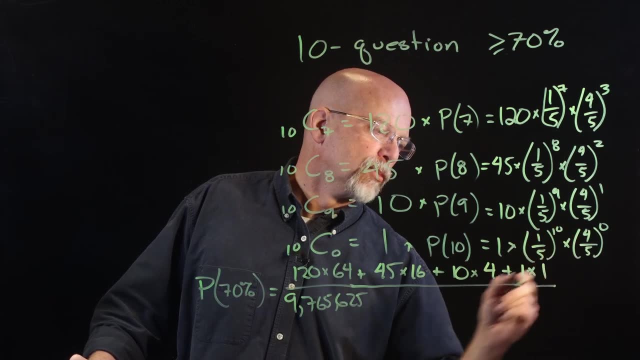 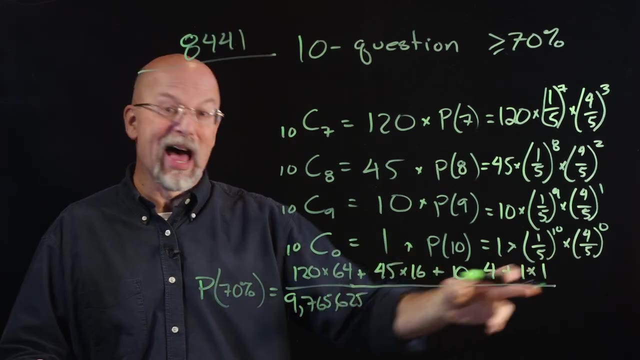 Plus, and then we've got 10 times 4 to the 1 is going to be 4.. Plus 1 times Uh, 1, right, And what we get is 8,441.. So there, that's a lot. 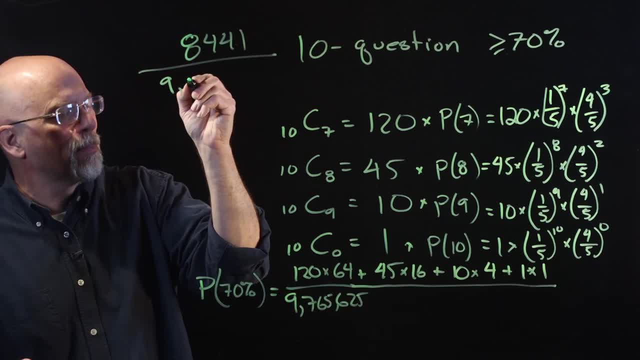 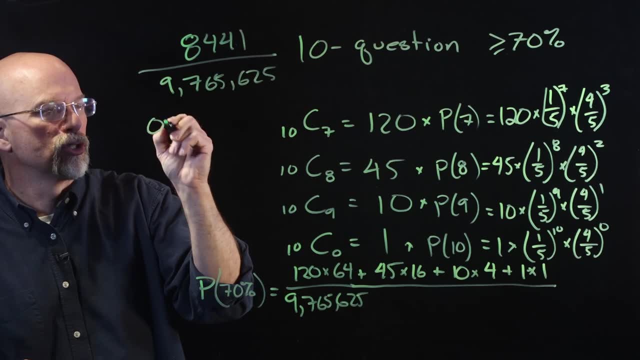 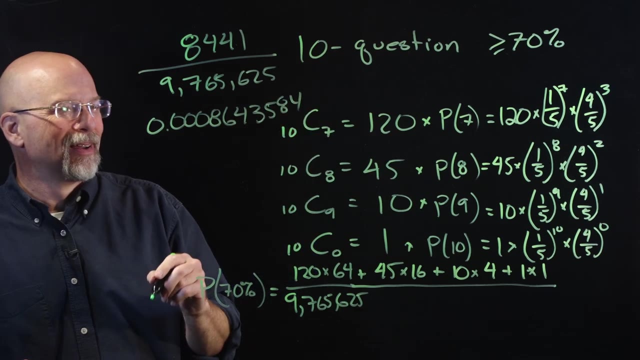 I mean, it looks like we've got a really good chance, right? Ah, then you divide it by 9,765,625.. And what you're looking at is 0.0008643584.. Well, let's just say that that's less than .09%. 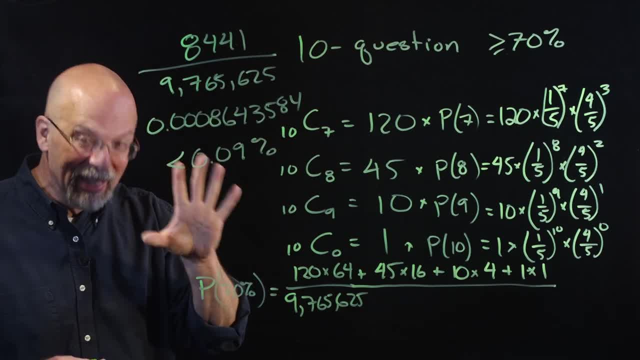 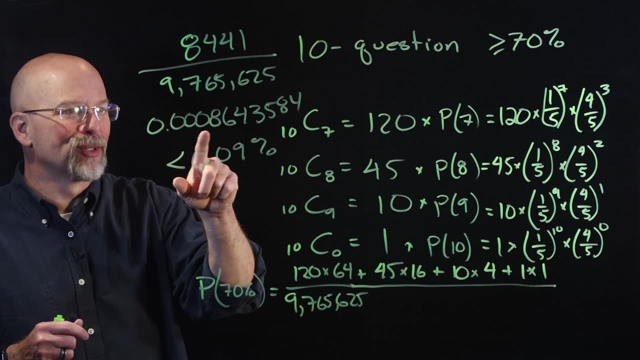 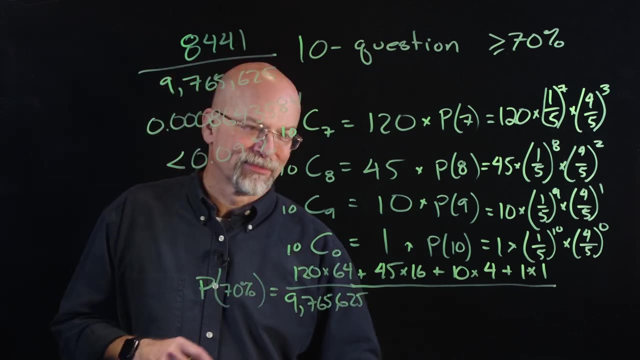 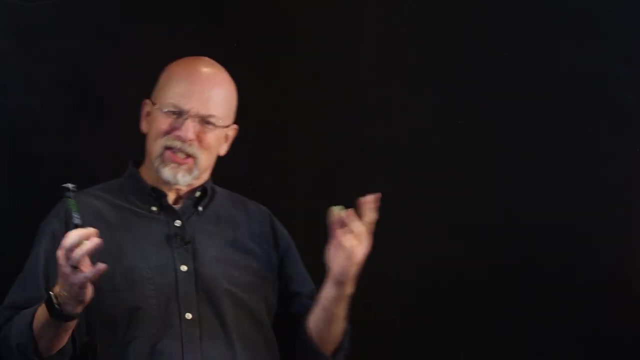 Are you willing not to study now? Less than .09%. You've got a probability of .000864, and so forth, in order to get a passing grade, if you're just going to guess. Well, since we're talking about low probabilities, let's talk about the most infamous of all low probabilities: a lottery. 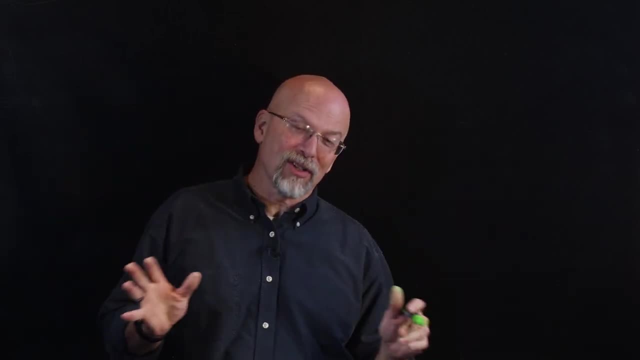 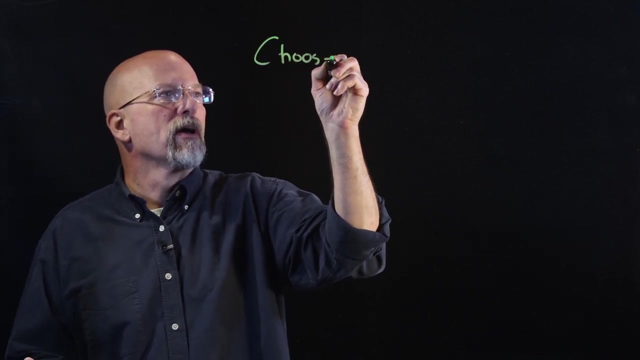 And for this we're going to talk about the most infamous of all: low probabilities a lottery, This particular lottery. I mean, there's a lot of lotteries all across the country that have this particular format. What you're doing is you're going to choose 5 from 69, is it? 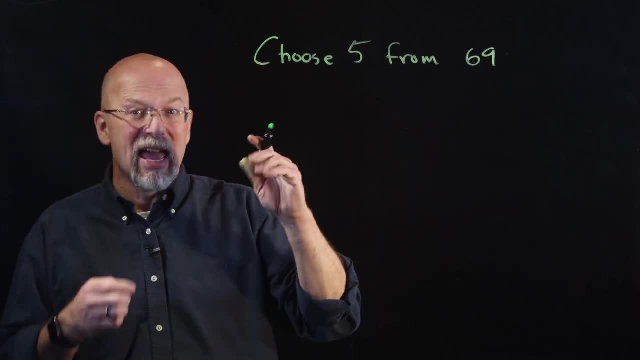 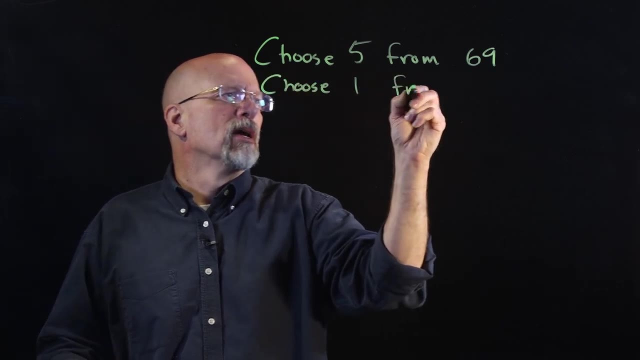 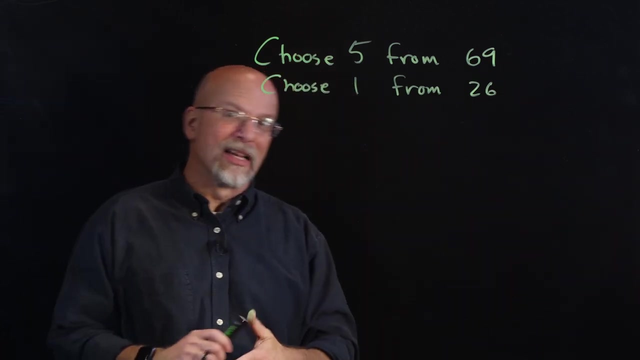 Alright. so you start out by choosing 5 from 69, and that will give you 5 of your numbers, And then you choose 1 from: is it 26,? I think it is Alright. And so the way you get the grand prize, the powerball, so to speak. 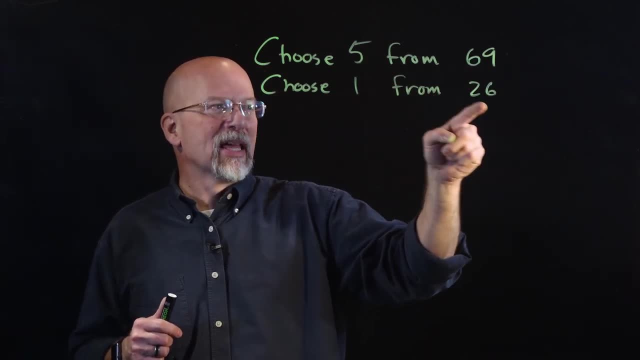 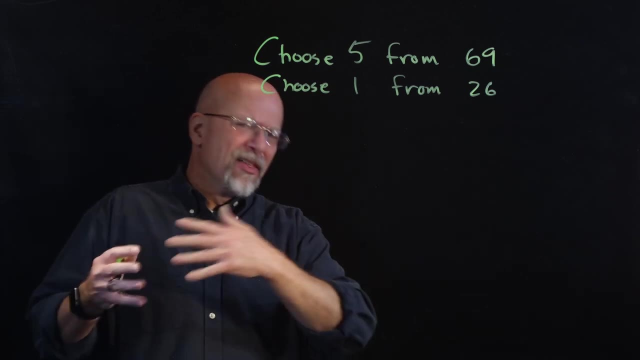 is to get all 5 of these right and that 1 right from the 26.. So there's no order, because once those numbers are picked, they're going to be sorted in numeric order. so you're not looking at any order here. 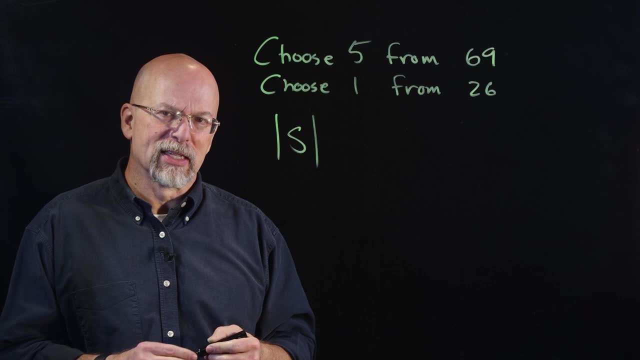 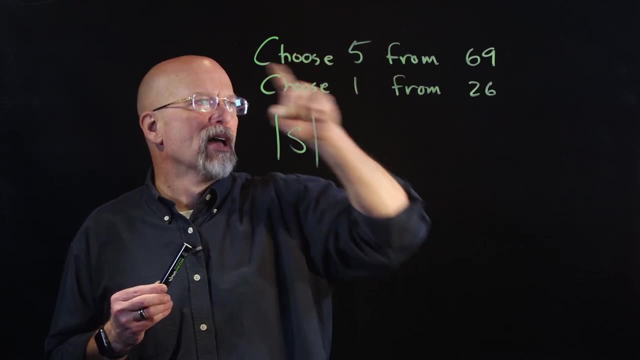 And so we need to figure out what our sample space size is right, The cardinality of our sample space. Well, what I'm going to do is I'm going to just figure out the cardinality of my sample space for the choosing 5 from 69.. 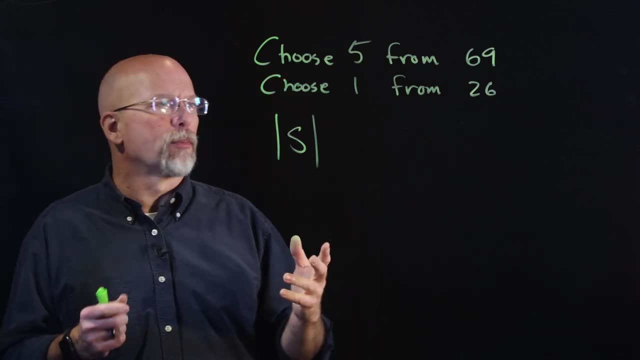 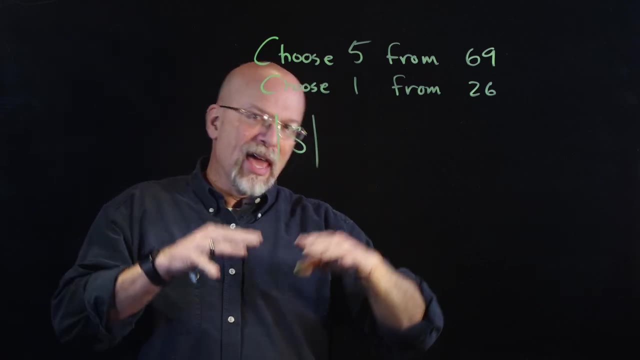 Why? Well, we'll see that whenever we're talking about the multiplicative rule for probability. once I figure out the probability for my different patterns from the 5 from 69, then I can multiply it by my different probabilities for whether I got this one right or I got that one wrong. 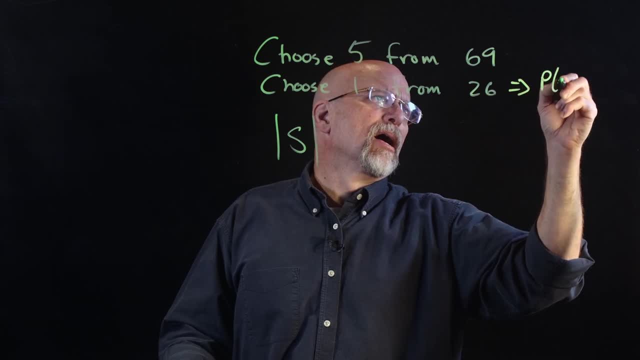 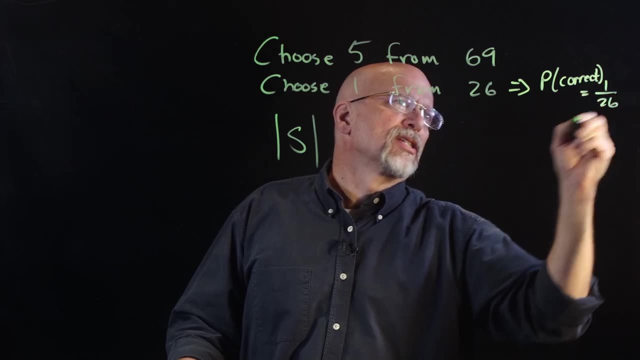 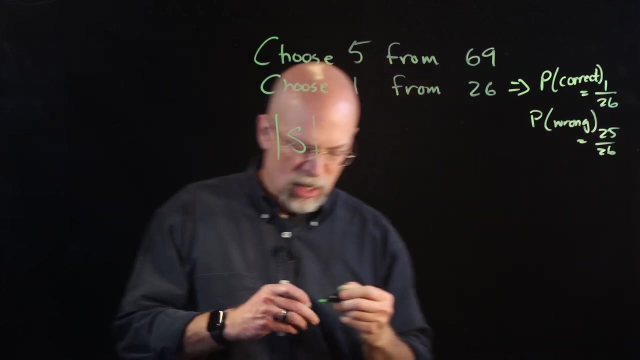 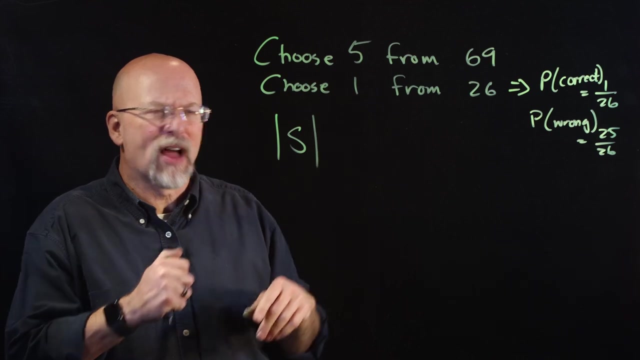 This one. it's pretty simple. The probability of Correct equals just 1 out of 26.. But the probability of wrong is equal to 25 out of 26.. So once I figure out my probability for the top bit, you know how well I picked 5 numbers from 69,. 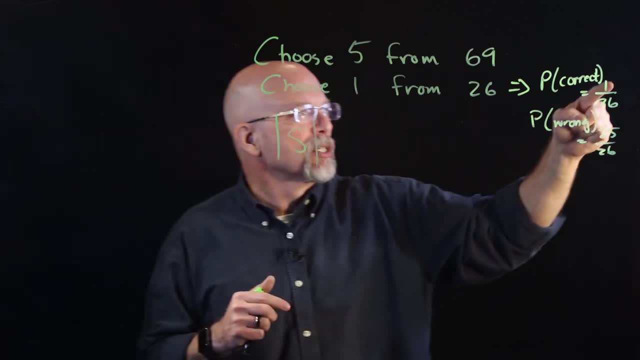 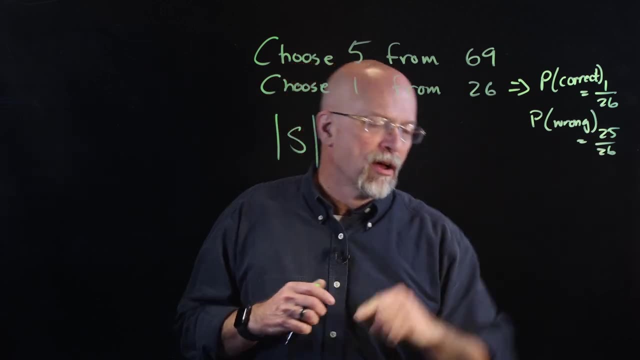 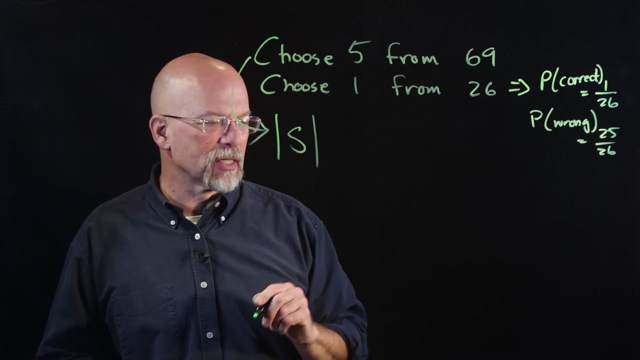 all I need to do, since I need to get both of these, is simply multiply it by either 1 over 26 for the correct or 200.. 200.. 25 over 26 for the incorrect. All right, So let's figure out what our sample space is, just from the 5 out of 69.. 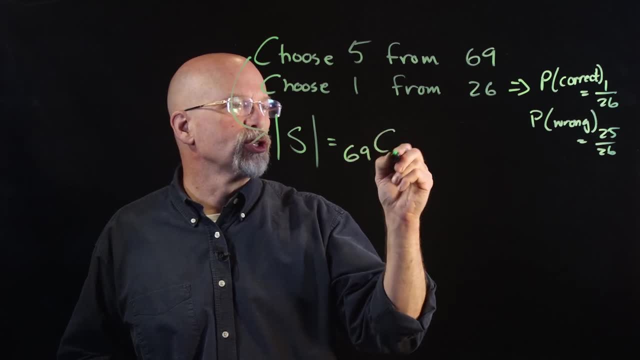 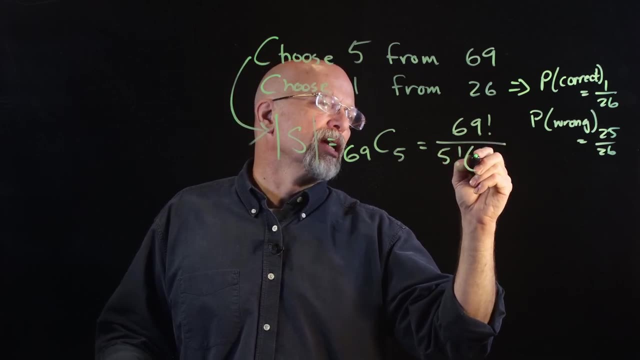 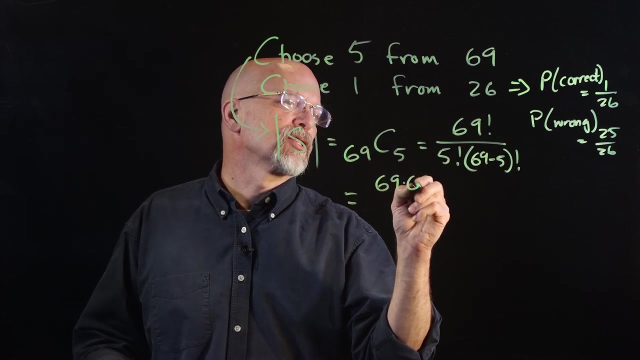 Well, the sample space is just going to be 69 choose 5.. Well, that's equal to 69 factorial over 5 factorial And still in the denominator you're going to have 69 minus 5 factorial. So this guy is going to be equal to 69 times 68 times, 67 times 66 times. 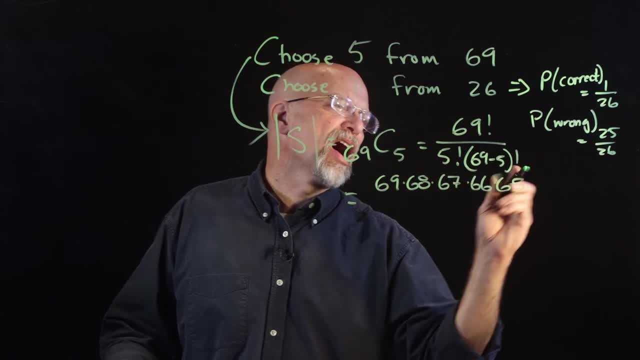 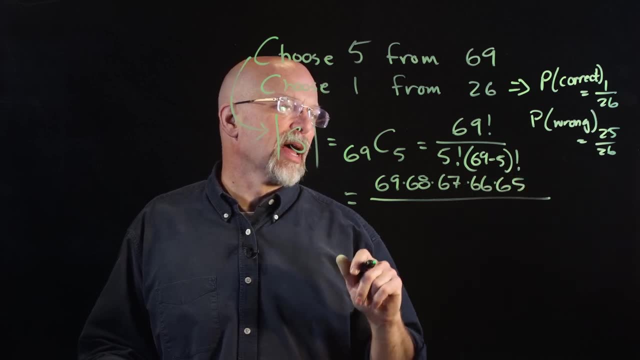 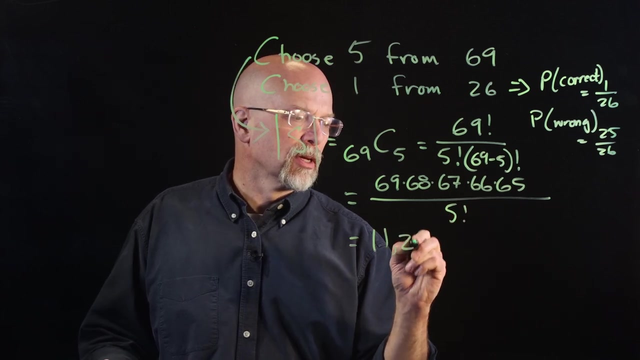 68 times 67 times 66 times 65, because 69 minus 5 is 64, so it cancels out all of the integers multiplied after 65. And then you divide it by 5- factorial right, And the result is going to be 11,238,513. 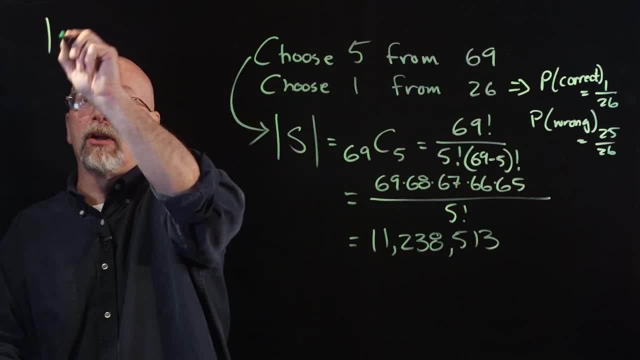 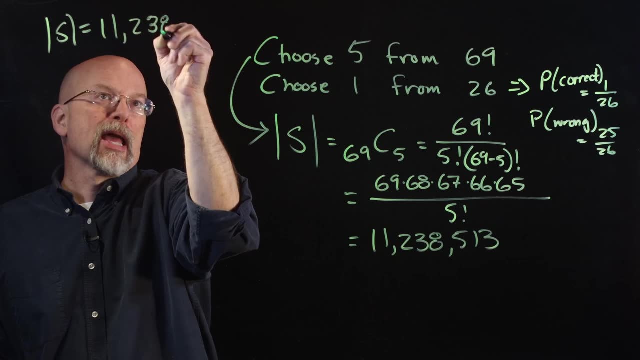 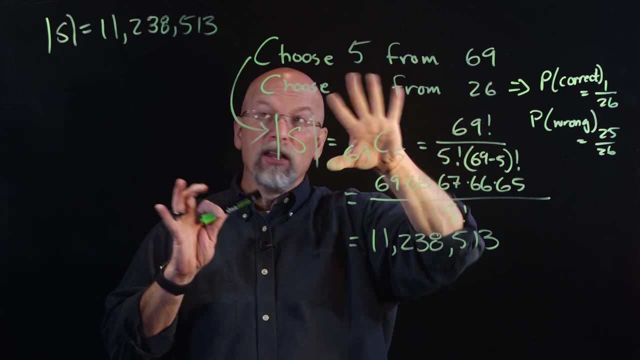 So that is our sample space And, in fact, what I'm going to do is I'm going to write this up here. The sample space for the choose 5 from 69 is 11,238,513.. All right, Now, if we want to get it so that all of these are right. 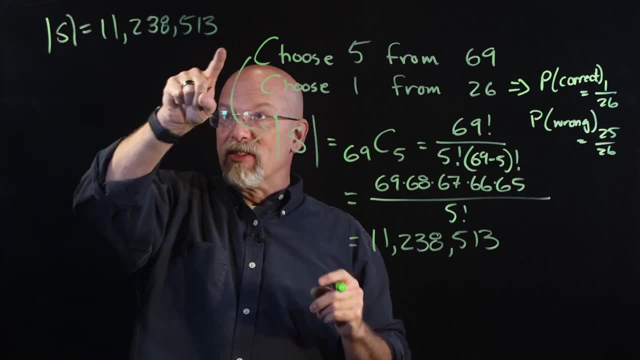 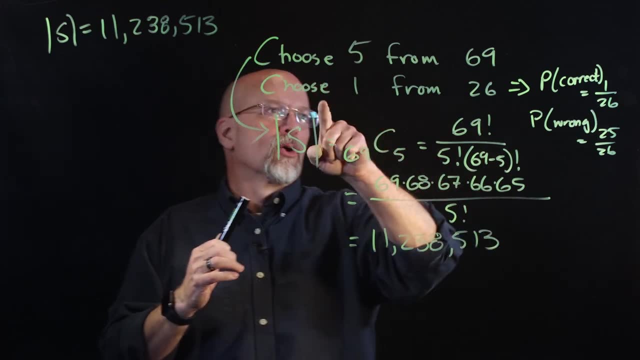 then I have one way in this sample space. One way, All five numbers are correct. One way in that sample space in order to get it correct And in order to get the Powerball correct, I also have to get this Powerball. 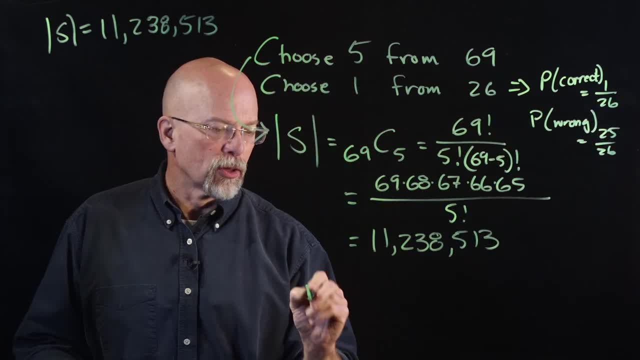 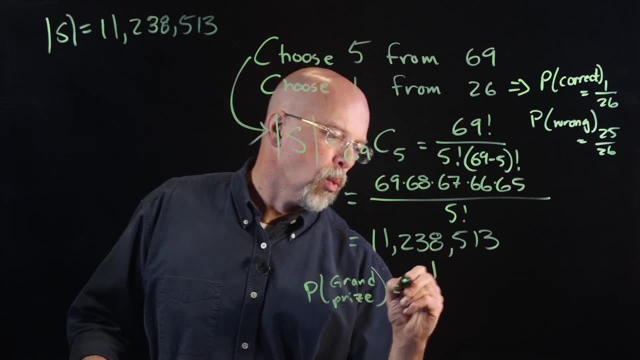 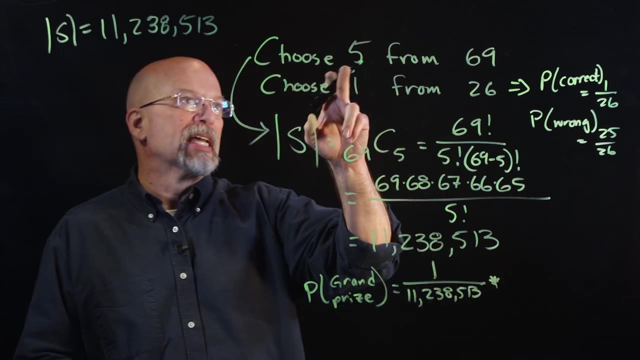 I have to get the 1 out of 26.. So the probability of the grand prize is equal to 1 over 11,238,513.. All right, That's getting the exact set right of the 5 from the 69. 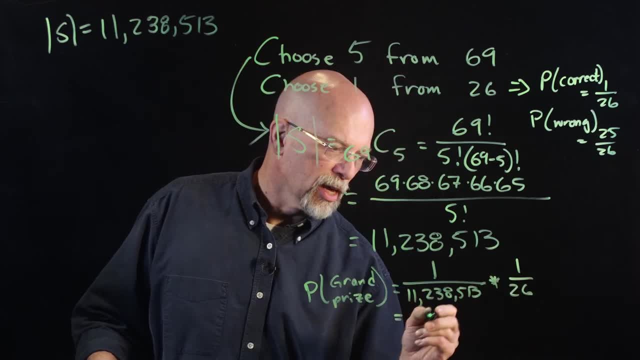 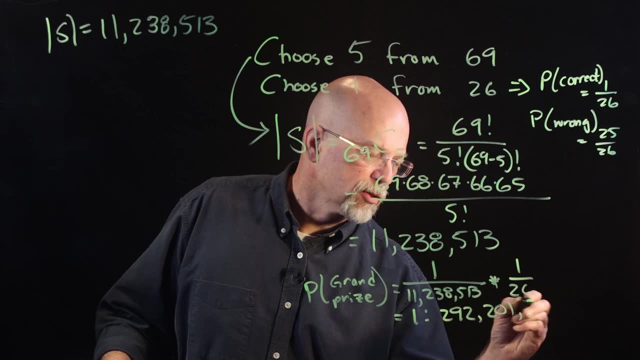 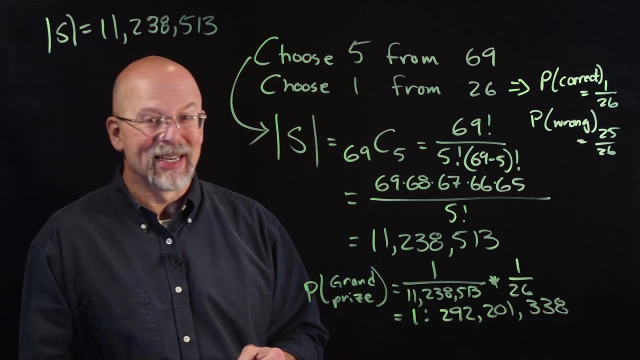 times the 1 over 26,, which is equal to the odds being 1 to 292,201,338.. Well, those are pretty awful numbers. What if we decide that it's okay to not get the grand prize and instead just get one of the top prizes? 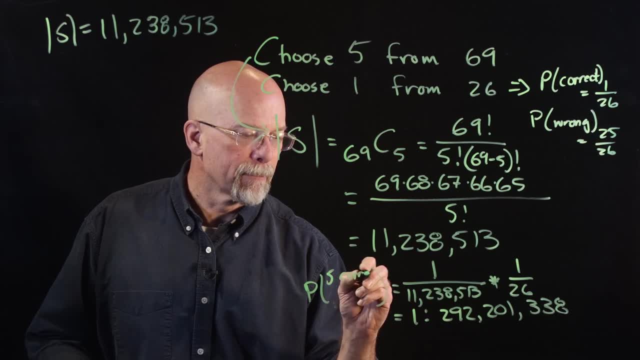 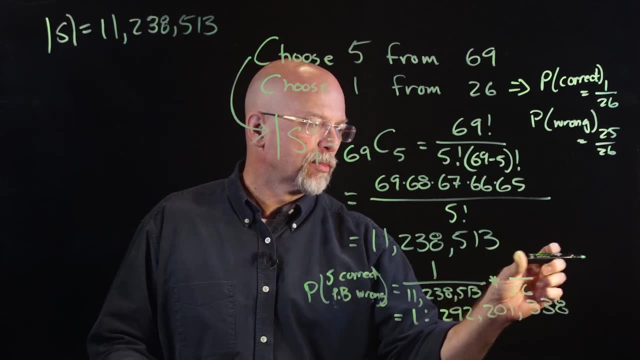 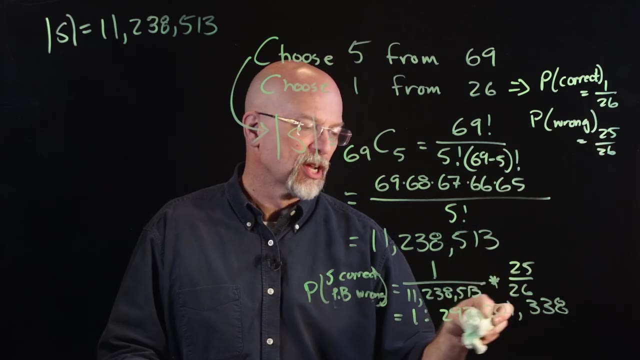 where I get 5 correct but the Powerball wrong. Well, in that case, I'm just simply going to replace that 1 with a 25.. Why did I do that? Because I have 25 wrong numbers to pick out of the 26. 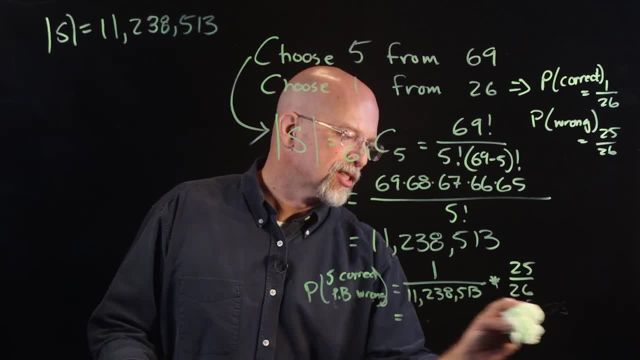 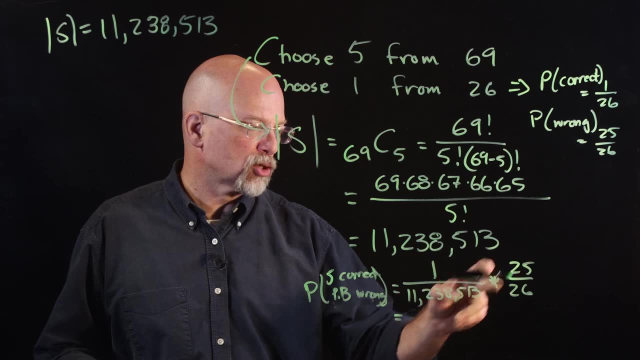 that were available to me. What are the odds then? Did that improve much? Well, let's see If I do this calculation, if I do this multiplying 25 over 26 times the 1 over 11,238,513,. 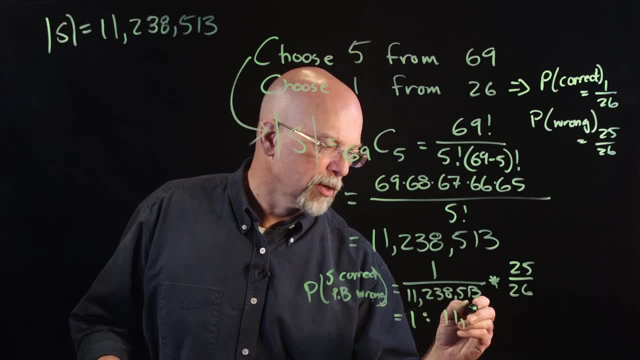 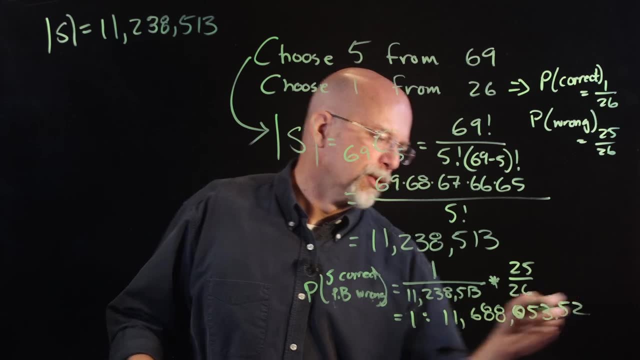 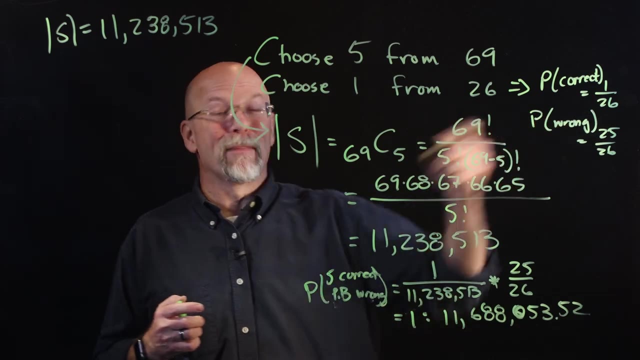 I get odds of 1 to 11,688,053.. That's like .52.. All right, So not an integer, Not quite an integer, And these odds are better than if I picked the 26.. I picked 1 out of the 26,. 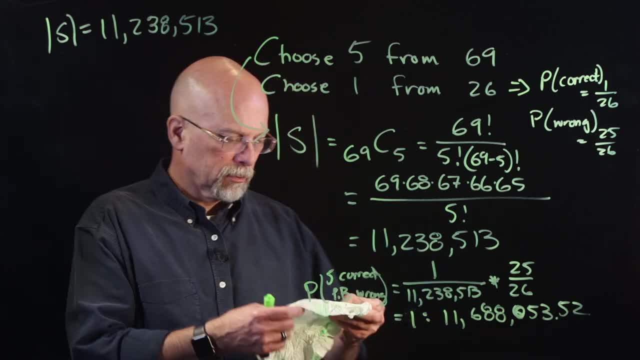 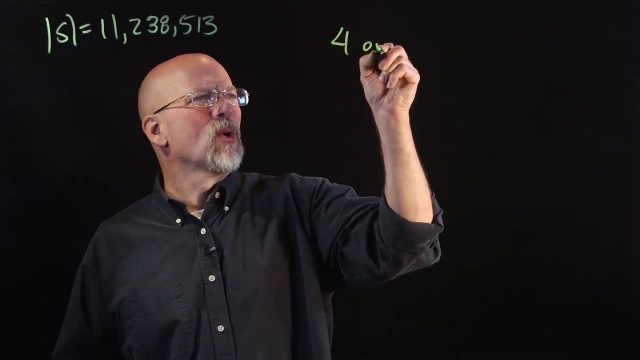 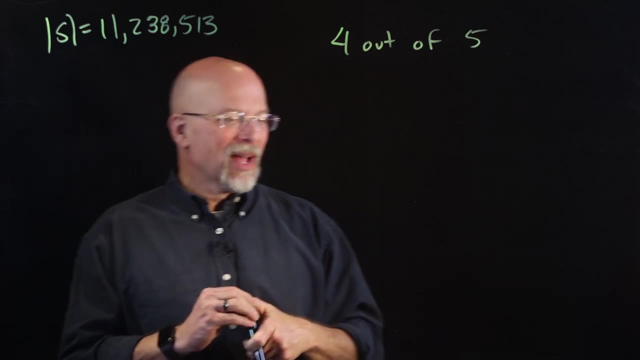 but they're not a whole lot better. So what if I lower my sights and I'm okay with 4 out of 5?? All right, Lower winnings, but the odds are better, right? Well, if that is the case, 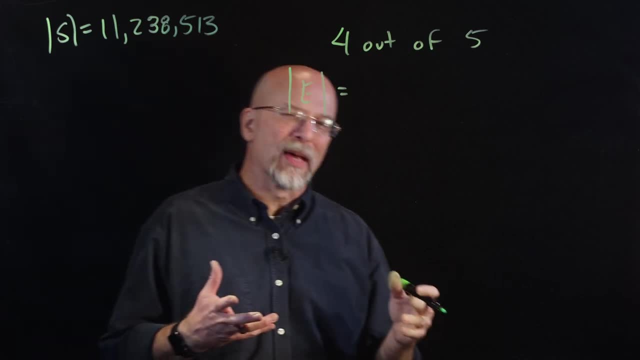 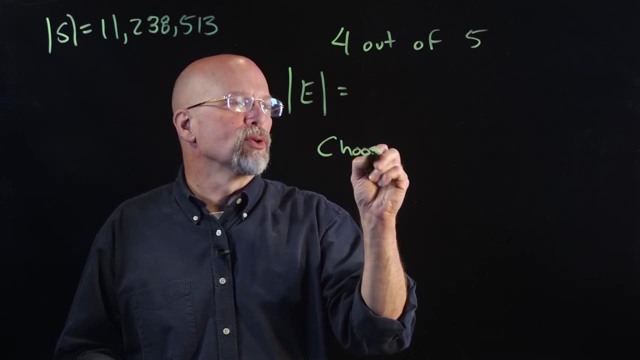 let's first look at what the cardinality of our event space is right, And so, in this case, what we're looking for is to, first of all, we need to choose which number is wrong, And I know that kind of sounds funny. 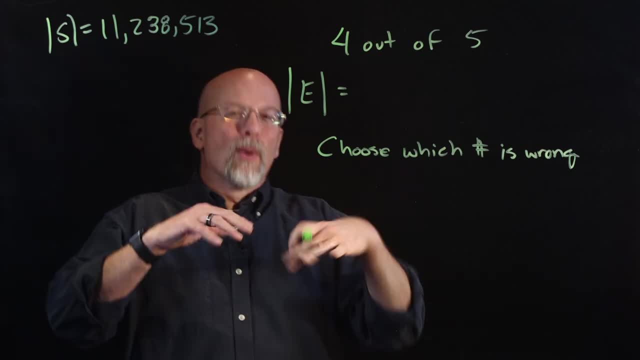 It almost sounds like: well, if I knew what number was wrong, then I'd choose it right. No, What we're talking about is probability. We have to figure out which one of those five numbers is going to be the wrong one. 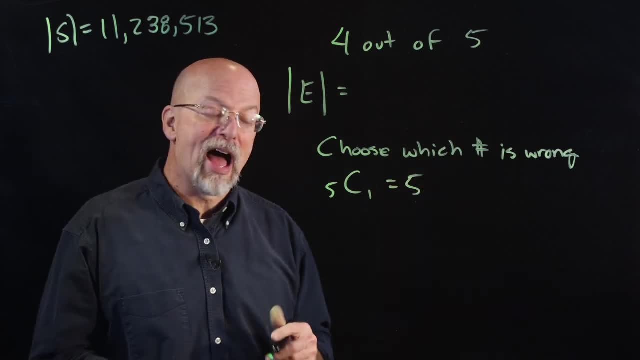 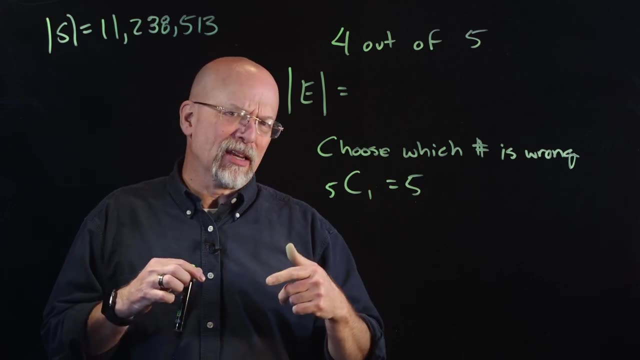 And so this is 5. choose 1,, which is just equal to 5,. right Now that we've figured out which one of the positions it could be, any one of those numbers that's wrong. now we need to figure out. 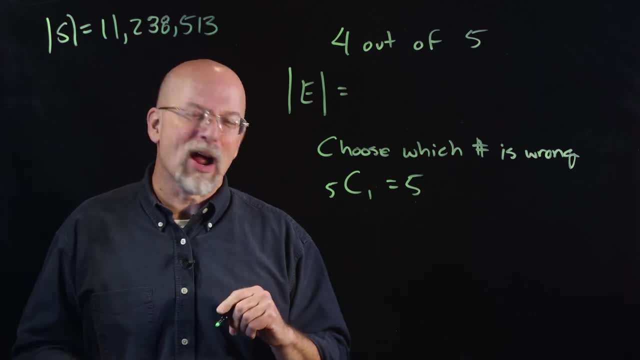 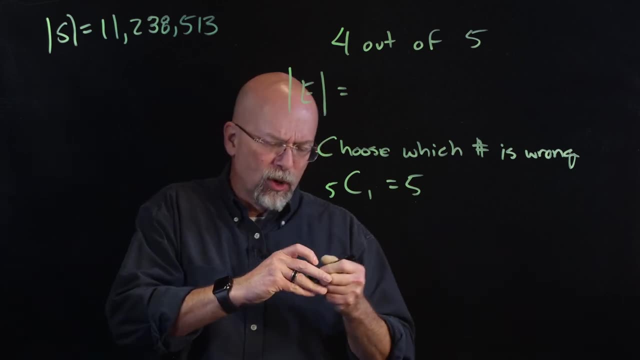 which wrong value it is going to have. Well, how do we figure out which wrong value it's going to have? Well, it has to pick from one of the 64 that's left over from the right. In other words, we've got 69 numbers total. 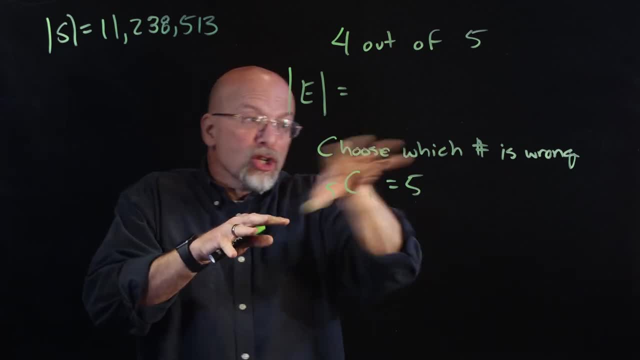 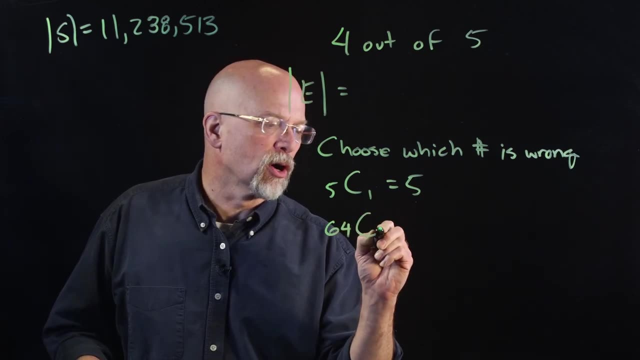 Five of them are correct. When I get to choose which number is wrong, I have to choose it from the number of incorrect ones, So that's going to be 64. choose 1, which is, of course, equal to 64.. 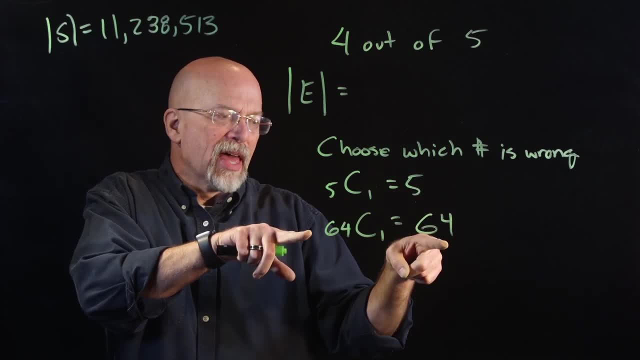 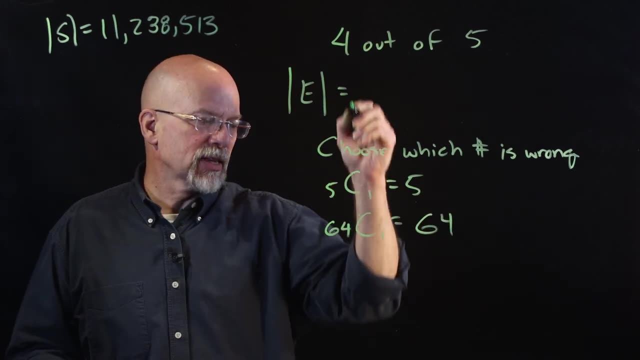 And so first picking out which one is wrong, then picking out what wrong value it's going to have, is 5 times 64.. That means that our event space is just simply 5 times 64, which is equal to 320.. 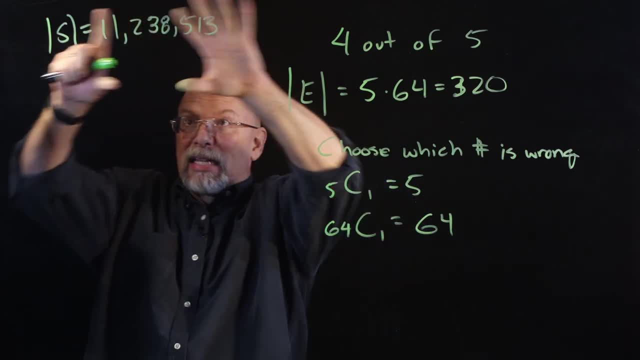 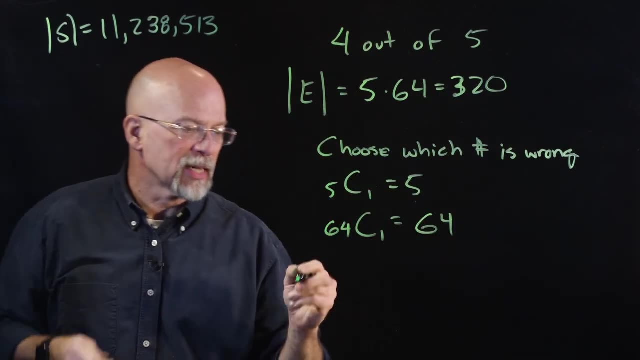 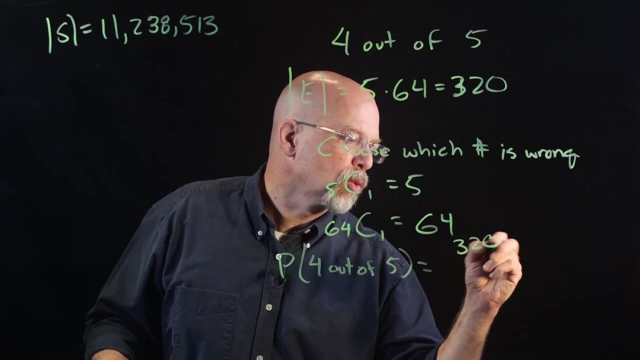 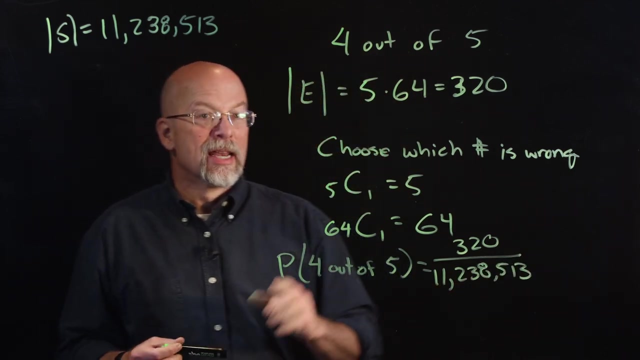 So that means that, out of my entire sample space, my event size is 320, which means that the probability of 4 out of 5 is equal to 320 over 11,238,513.. All right, Now, this doesn't talk about the Powerball. 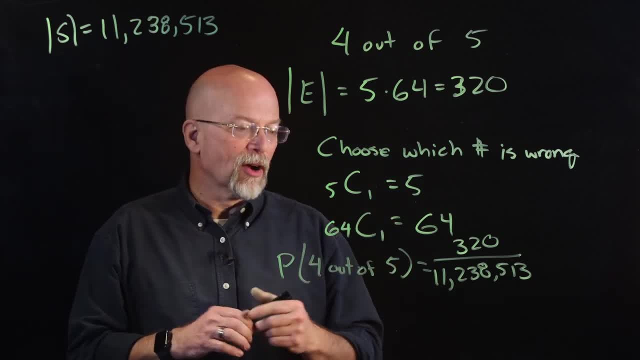 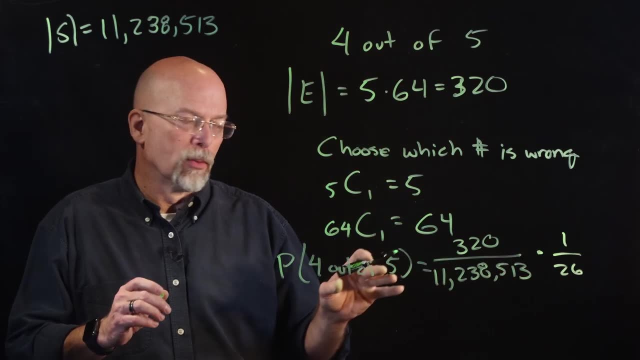 Remember I said the Powerball was separate. Well, if you want to figure out with the Powerball, if you get the Powerball correct, that's times the chances- 1 out of 26,- of getting the Powerball correct. 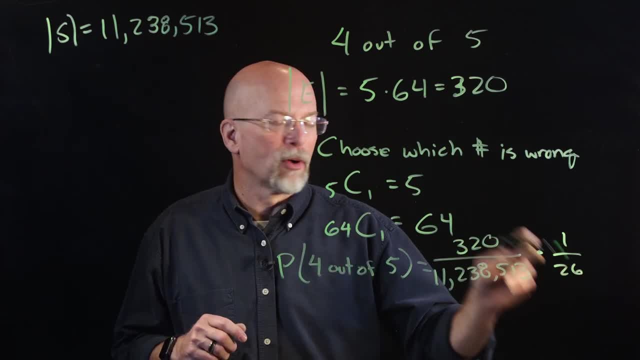 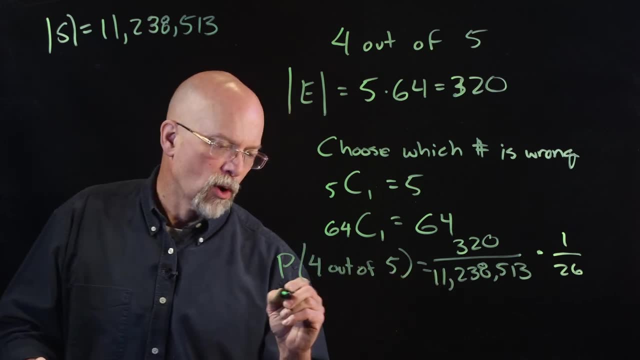 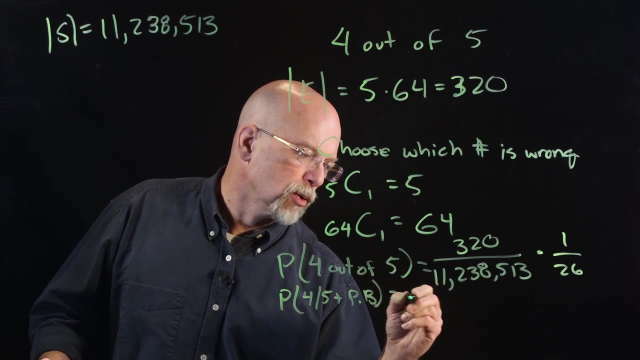 If you're okay with getting the Powerball incorrect, then you multiply it by 25 over 26.. And what this gives us is that for the P, 4 out of 5 plus Powerball is correct. that's equal to- and I did this before- 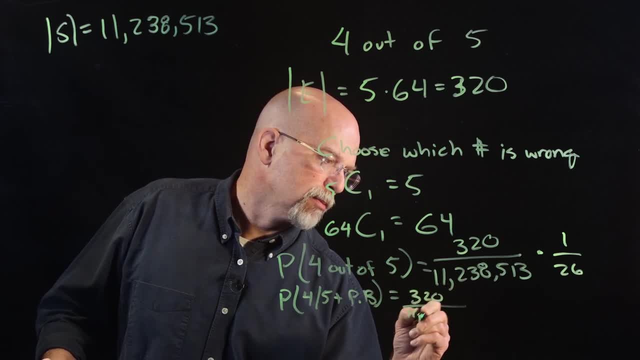 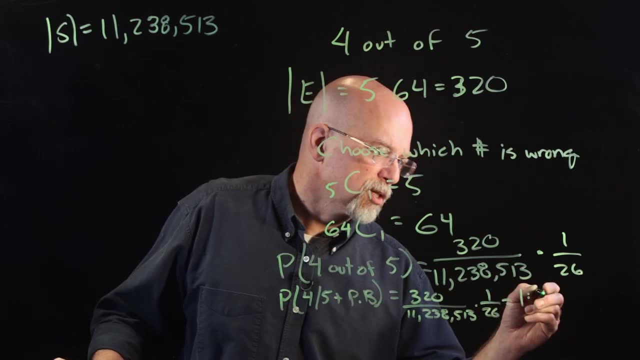 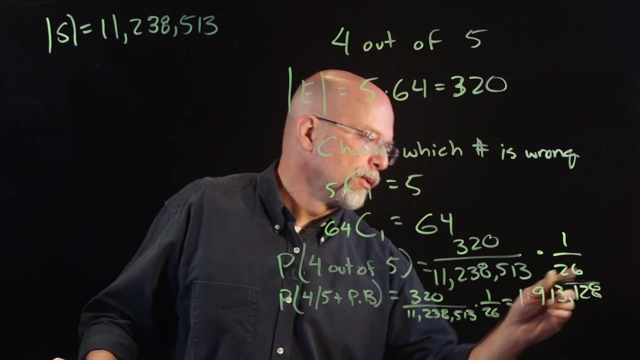 so it's 320 over 11,238,513 times 1 over 26,, which is going to give you an odds of roughly 1 in 913,129.. Whoops, I said 9,, wrote 8. 129.. 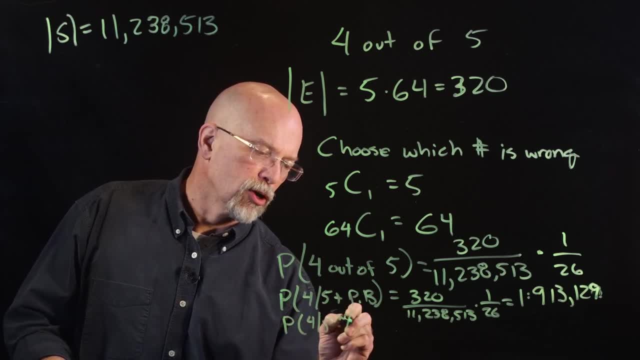 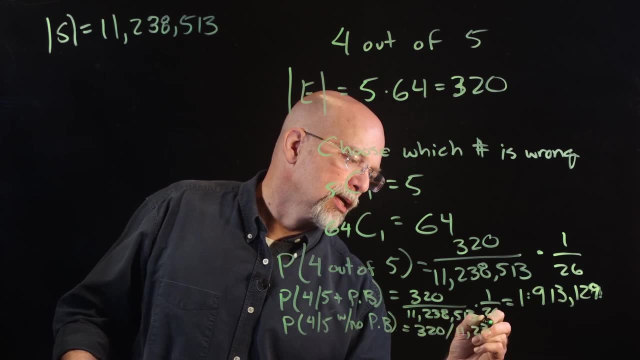 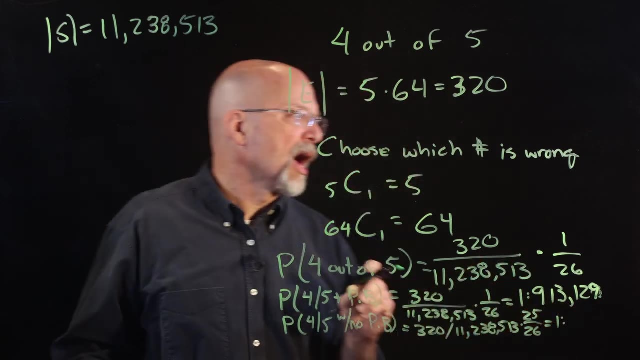 Now the probability of 4 out of 5 with no Powerball. that's equal to the 320 divided by 11,238,513 times 25 over 26,, and that's going to give you odds of- and I hope you can still read this: 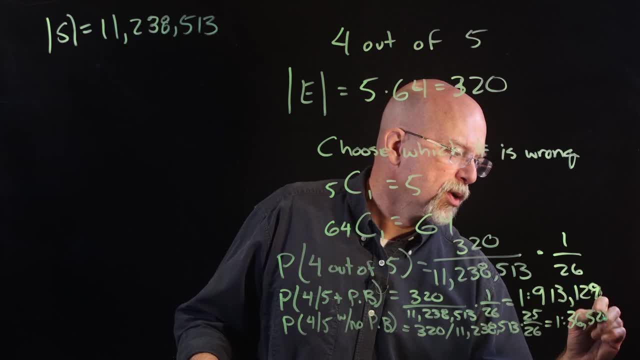 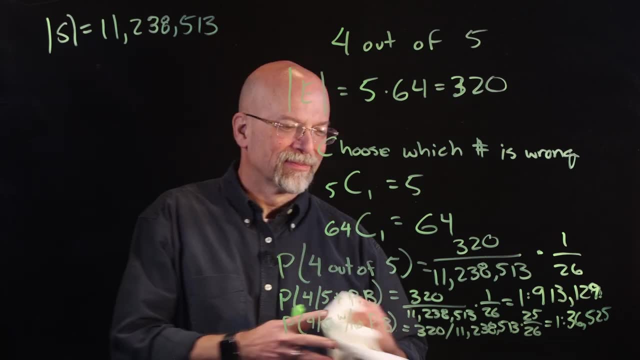 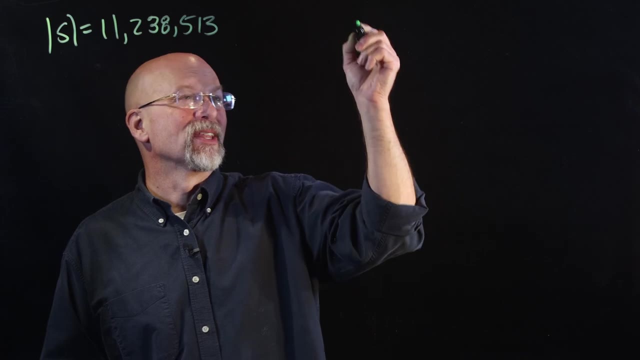 36,525.. All right, Much better odds. Still not great, but much better odds. Let's lower our sights even further, and I promise this will be the last one. What if we're okay with 3 out of 5?? 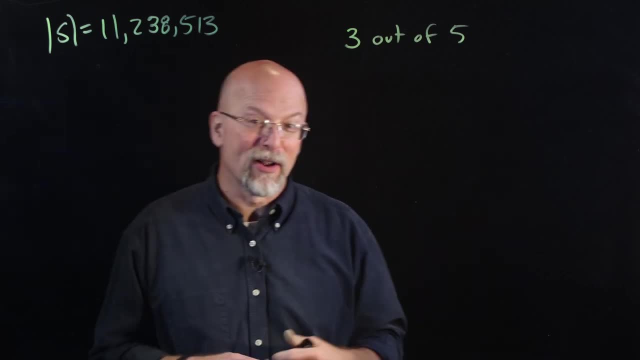 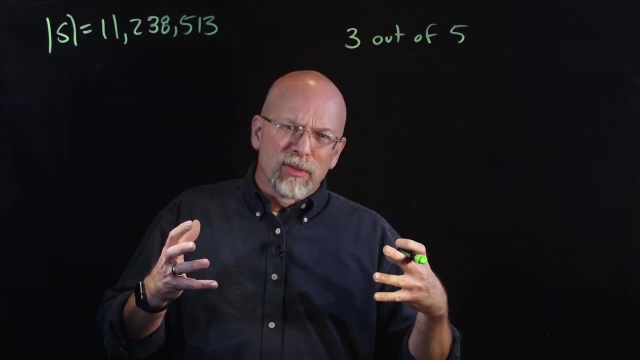 Well, first of all, we had to figure out what the size of our event subset is. right, And our event subset in this case is going to include all of the possible combinations where we chose exactly two numbers to be wrong, And so we've got 5, choose 2.. 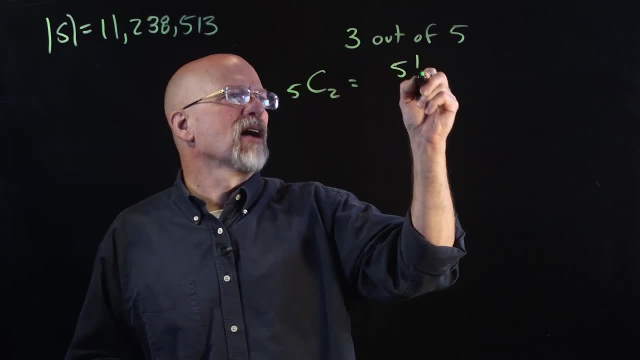 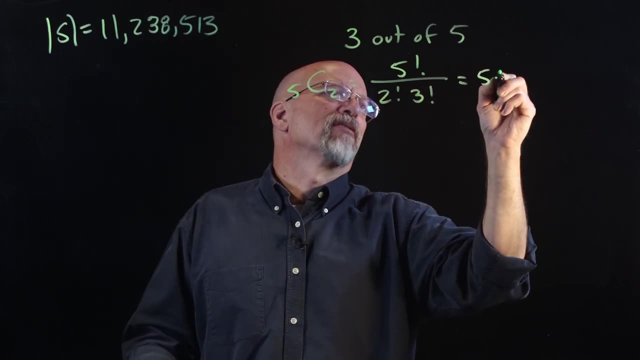 5 choose 2 is 5 factorial over 2 factorial times 3 factorial, which is going to give us what 5 times 2, which is equal to 10.. So there should be 10 ways to choose 2 out of 5.. 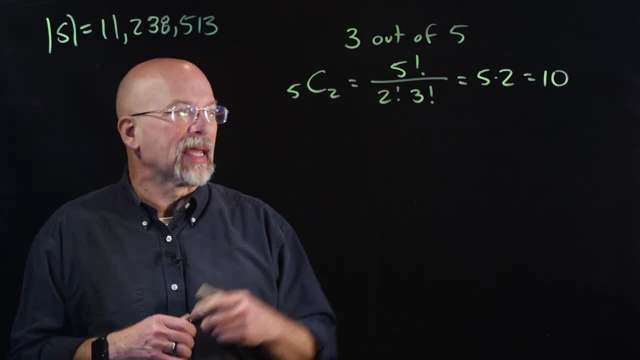 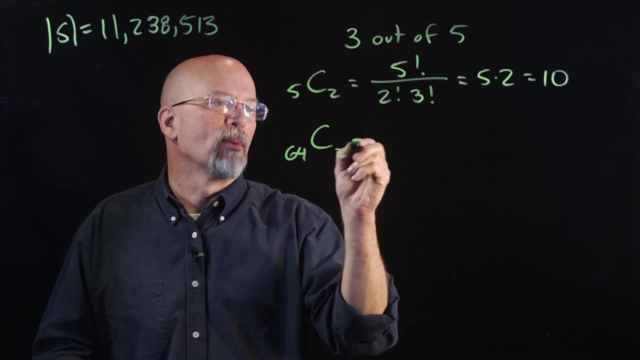 Now we need to figure out which values we're going to make as incorrect. Well, the way we need to do that is we need to take the 64 incorrect values and we need to choose 2 of them. So we've got 64 factorial. 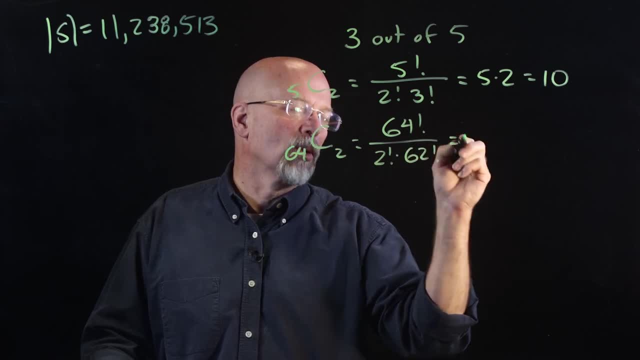 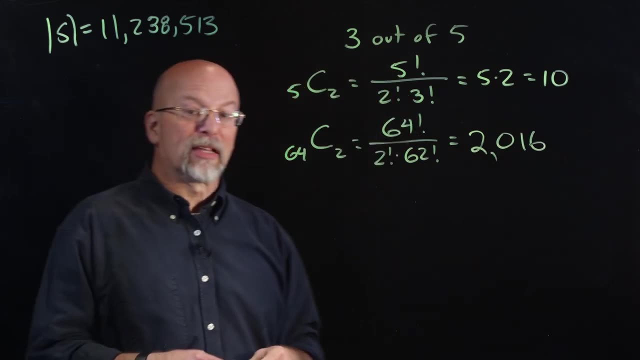 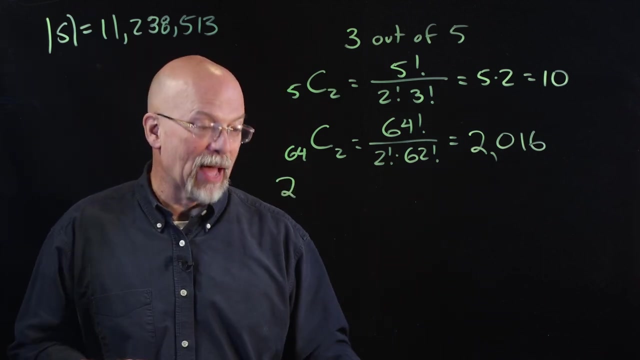 over 2 factorial times, 62 factorial, which is going to give us 2016.. So there are a lot of ways to pick those 2 wrong numbers right? Well, that means that there are actually. what that means is that the size of our event subset. 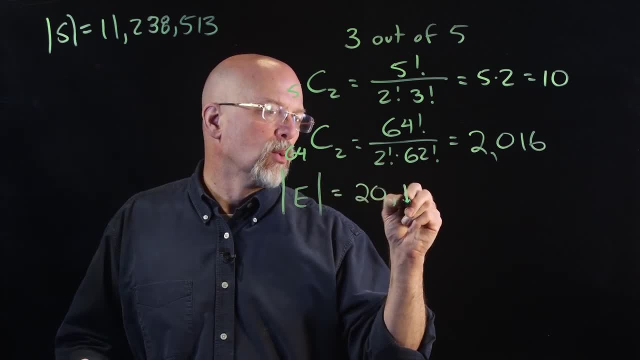 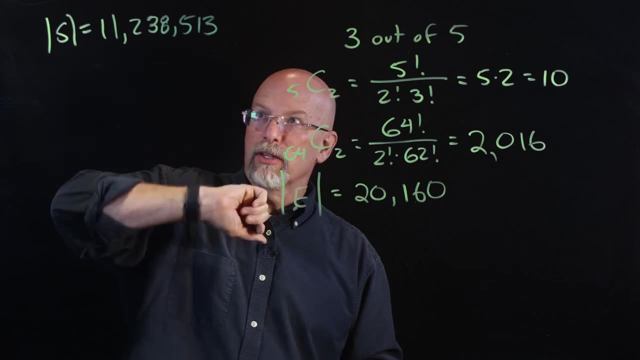 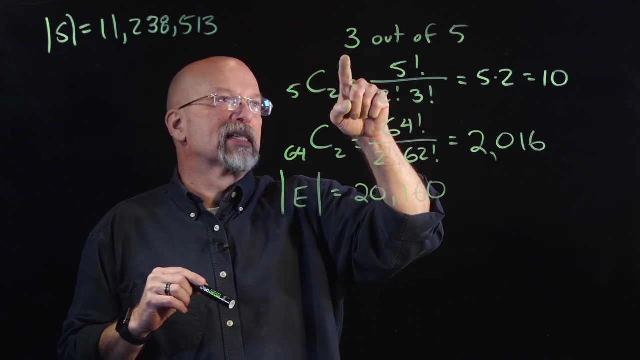 is equal to 20,160.. So there are 20,160 ways out of this total, right up here 11,238,513.. There are 20,160 ways to pick exactly 3 out of 5.. That gives us a problem. 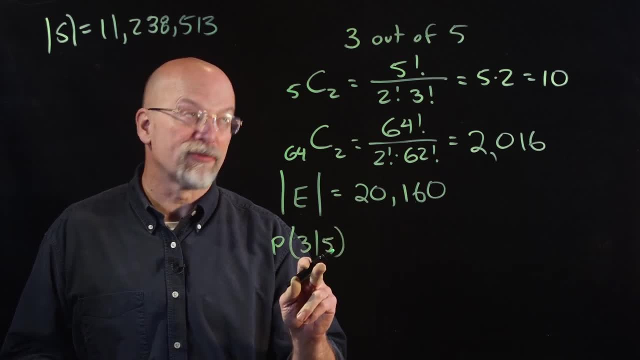 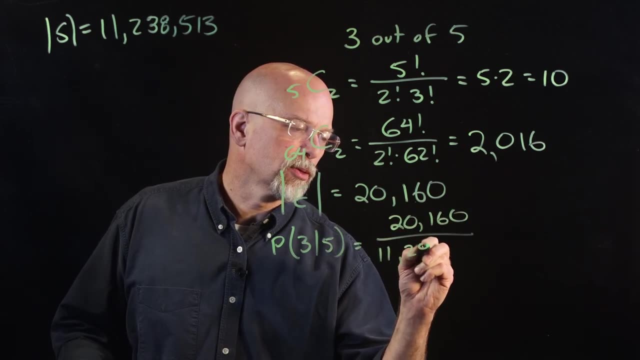 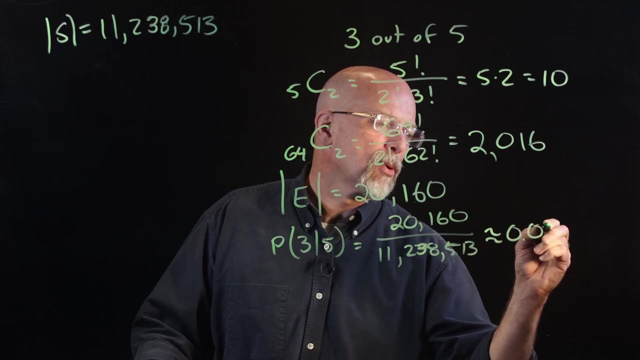 That gives us a probability for picking just 3 out of 5, right of 20,160 over 11,238,513, which is just about equal to 0.0018.. What this means is we've got twice the chance of picking 3 numbers out of 5.